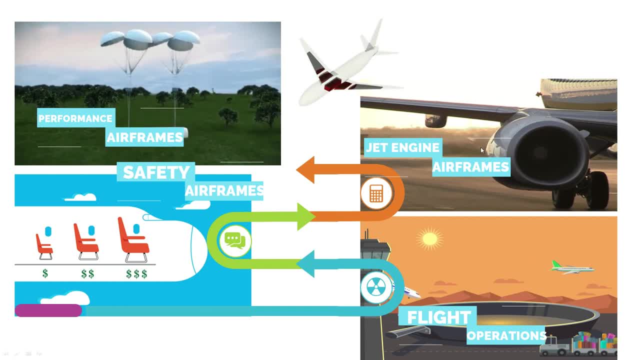 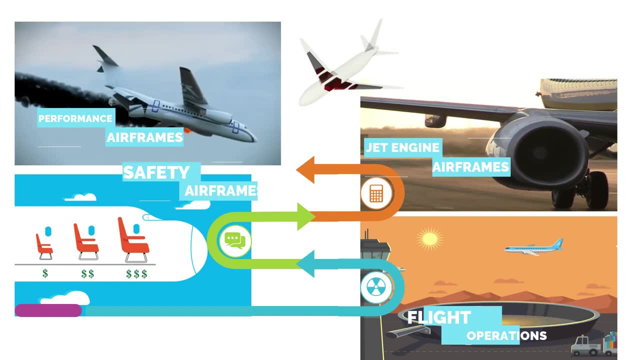 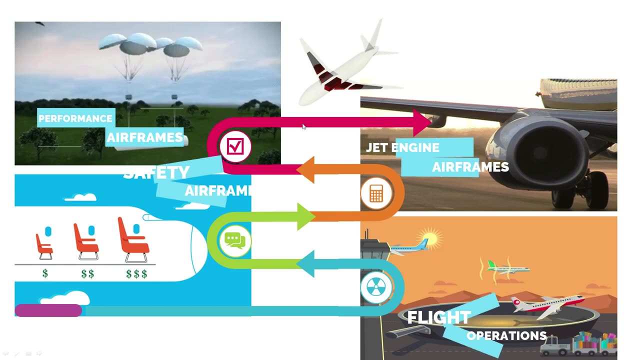 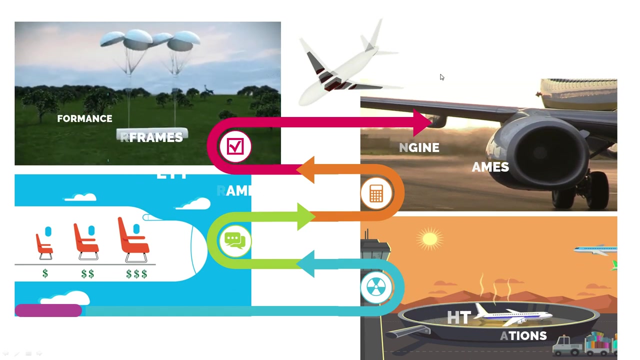 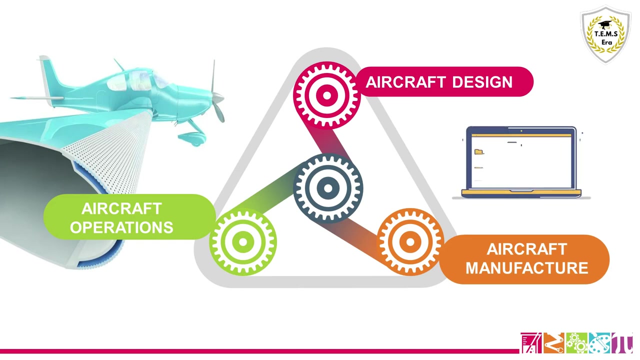 performance of the aircraft which directly or indirectly considered as structural material, Safety, critical air from components needed, as I've seen, the key concern for an advanced material developments such as properties, manufacturing availabilities, fabrications and also cost. So all those are connected directly or indirectly by the engineers working in the field of 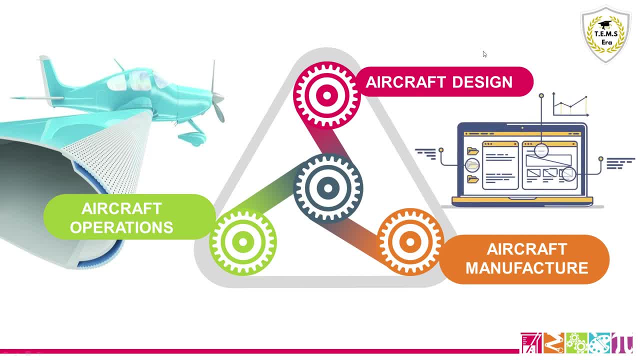 aircraft design, aircraft manufacturing and aircraft operations. Now, talking, all those factors, this advanced material have a great, great, great importance in improving the structural efficiency of the aircraft and Also the propulsion efficiency of an jet engines. now you might think how, by considering the material properties. now we'll talk about 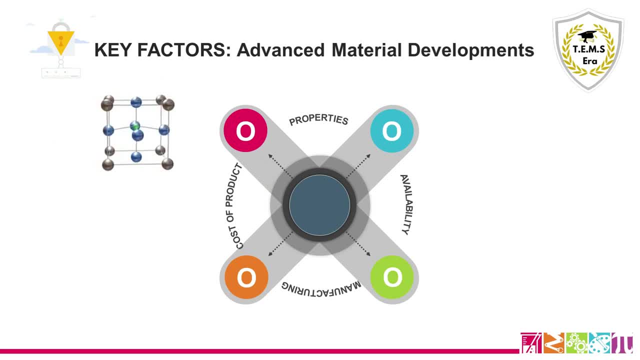 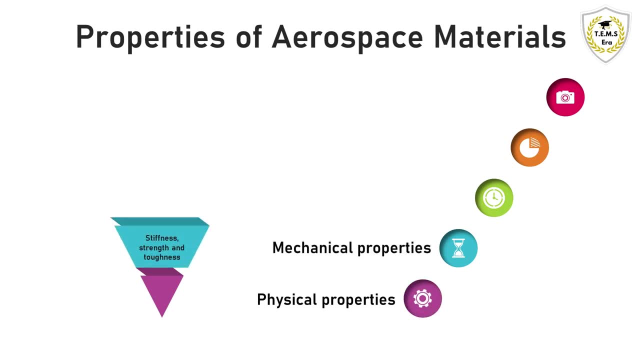 material properties that are important to aircraft, including physical property, for an example of density, mechanical property like stiffness, strength and toughness. chemical properties like corrosion or oxidation, thermal properties like heat capacity or a thermal conductivity, and talking about electrical properties- electrical or magnetic properties or conductivities- now the main. 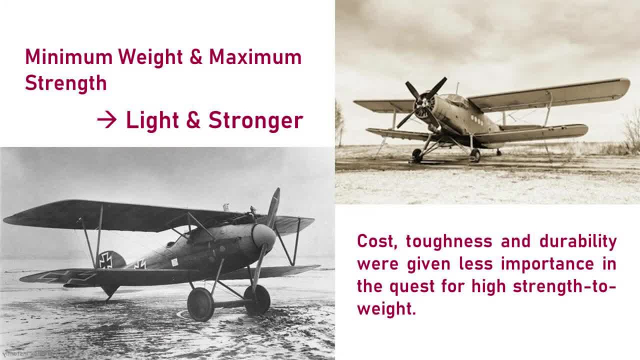 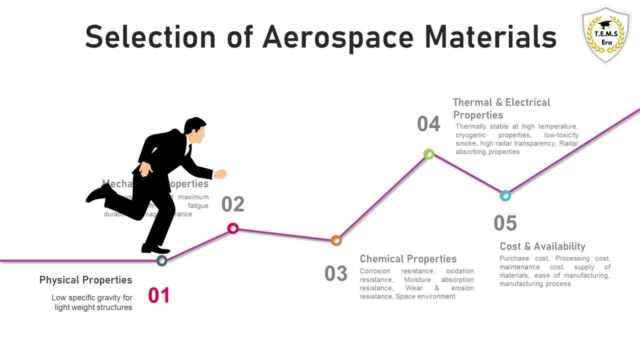 criteria for material selection for an earliest aircraft was minimum weight and the maximum strength, not talking about a physical property. the physical property Defines the density. now, when I'm talking about density, density Which is directly connected with an specific gravity- lower the specific gravity of the material, lower is a lightweight structure. 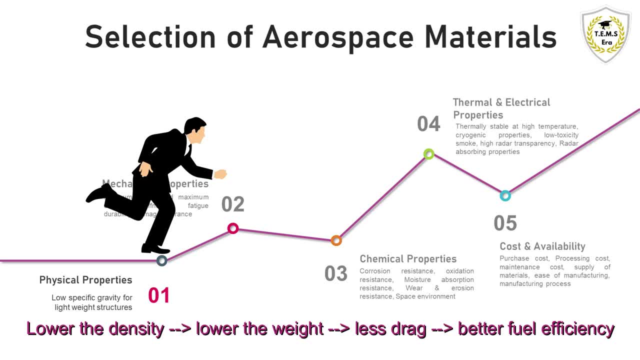 So once it is lightweight it is more more fuel economy. if the fuel economy is high then obviously the drag will be less. so both are directly or Indirectly correlated with each other. next, moving to this material property. now, material property, as you know, as I've said before, 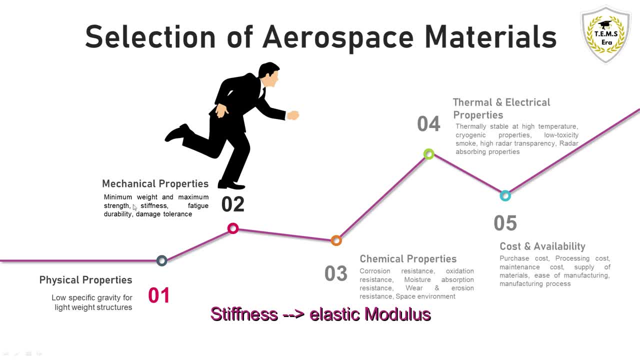 Stiffness. when I talk about stiffness, we need to keep in mind about the elastic modulus Strength. yes, strength, when we talk, you have to keep in mind about the yield and the ultimate strength of an aircraft and, apart from this, stiffness and the strength over some few more factors is also play a key role of. 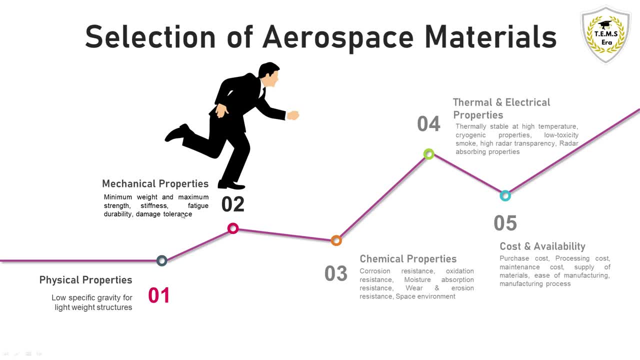 Fatigue. durability of what is fatigue durability? it resists against the Initiation and the growth of crack from various sources of fatty. it can be due to the stress, It can be due to the combination of stress and corrosion, thermal or even acoustic. Now another factor comes: a damage: tolerance. 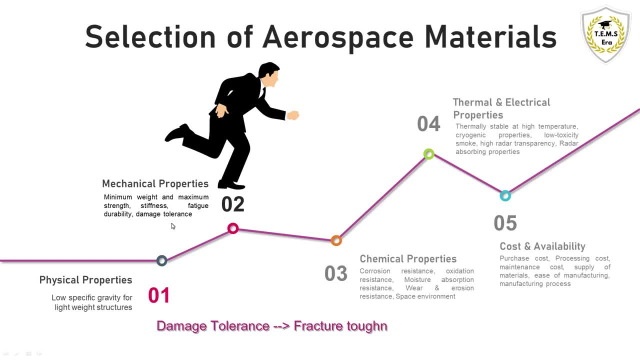 damage tolerance explains about. suppose a Maintenance officer is working on some particular component, now suddenly the tool get dropped over a particular Surface, maybe on a wing surface, maybe a fuselage- So it must have a capacity to resist an impact. so when a huge impact are undertaken by any 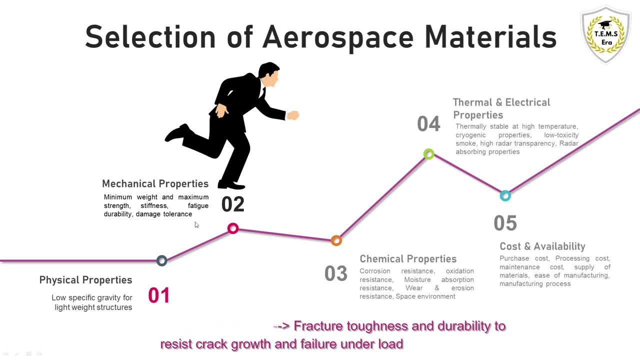 Structural component. it must resist the Crack growth or the failure under load. so it must resist such kind of phenomena. So this comes under the damage tolerance. So all those parameters need to consider under the mechanical property. Moving to the next, was a chemical property. chemical property as it says about the corrosion resistant. 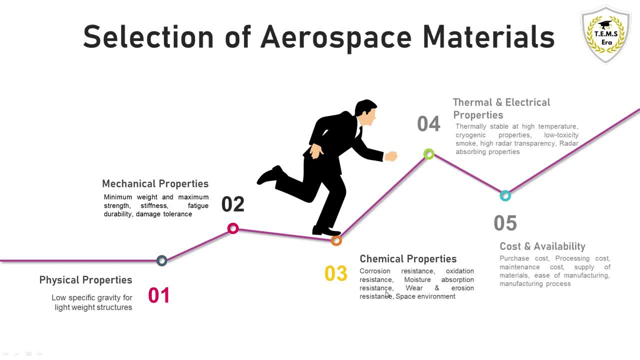 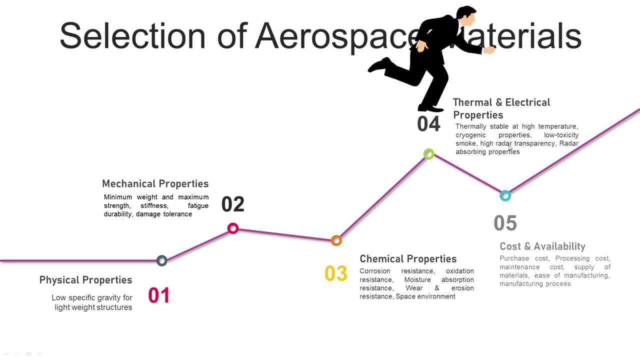 oxidation resistant, moisture absorbing resistant, wear or erosion resistant In space environment, like you know, kind of ionized radiations and so on. So such kind of categories will fall under the chemical our property now moving to us thermal property. Not talking about thermal property- Yes, thermal the name is that you can understand the word- the present heat. 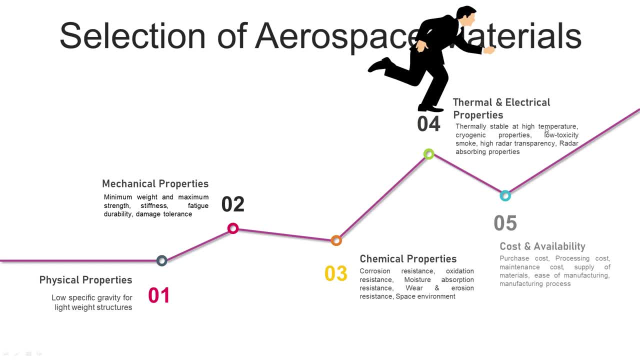 So thermal is stable at high temperature. and not only that, it must have high softening temperature, It must follow up with the cryogenic property And it must also allow for the emission of heat as well as the radiation, If the heat that is released is too high. 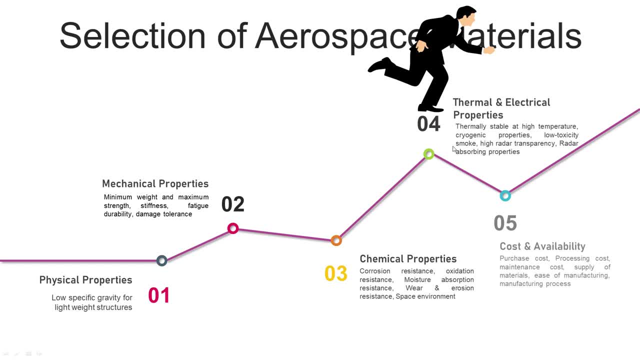 So it has to be fixed and it must not be damaged by the heat. So you can see the thermal properties, the thermal expansion properties, Even on a non or low flammable properties, low toxic smoke properties, all those properties will come under the thermal property. Now, moving to the next was a electrical or the 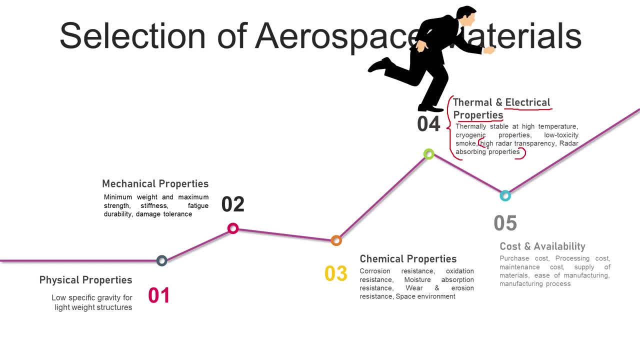 Magnetic properties now when we talk about the electrical and magnetic strikes. so such kind of phenomena must be observed for an aircraft before designing, then talking about high radar transparency- for an radar drone and even for some kind of military aircraft or some rather absorbing properties, like rather materials, like a ram material, rather absorbent. 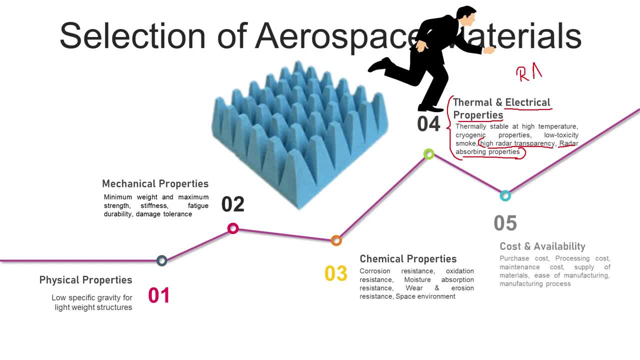 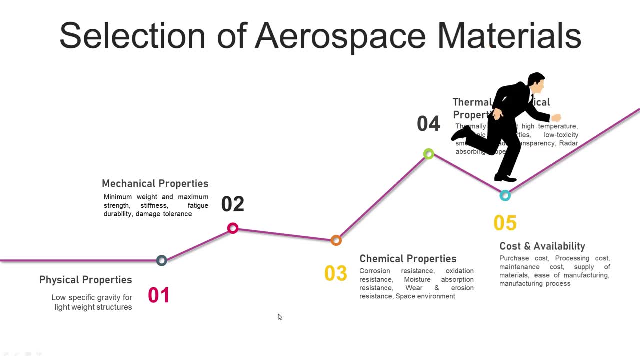 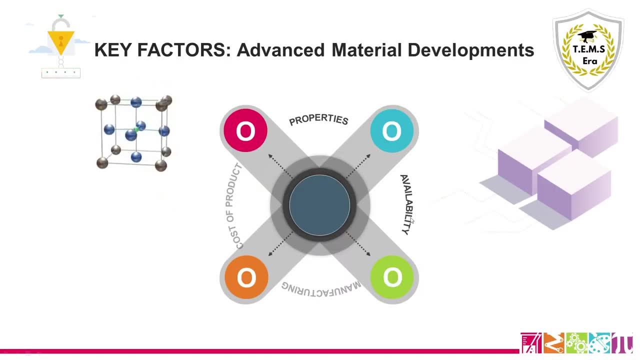 material. so such kind of things can be coming into this types of properties. now, moving to the next is the availability. now, what this availability is explains. it explains about the plentifulness of the material- uh, long term supply of the material. uh, better uh processing of the material. 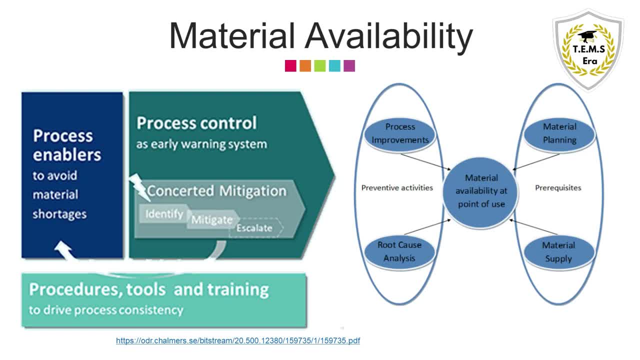 and uh, easily supplyable from one point to another point. so this is all about the availability. so once this availability also directly connected with the cost of the products, although if i talk about the cost of the products, yes, the cost of the products means the overall cost of the aircraft also. so this is what the metal availability is connected. 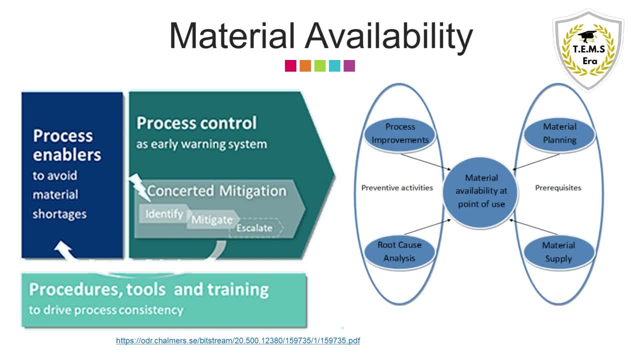 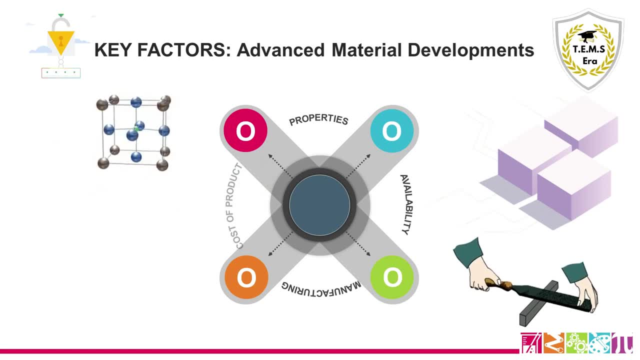 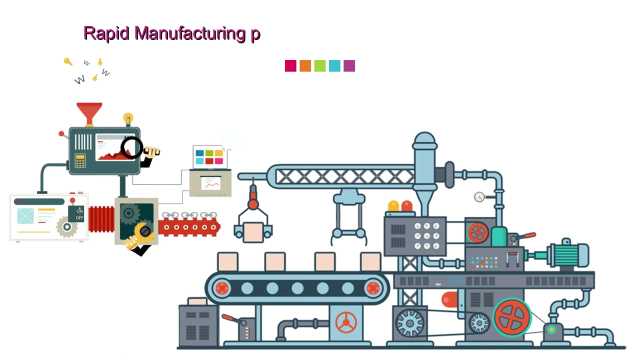 similarly, if i talk about this material, material manufacturing, yes, it is also readily available. it must be ease of manufacturing, low cost and rapid manufacturing processes readily available in the market. again, this, both availability and manufacturing, are connected with each other. so more the rapid manufacturing process, better large amount of. 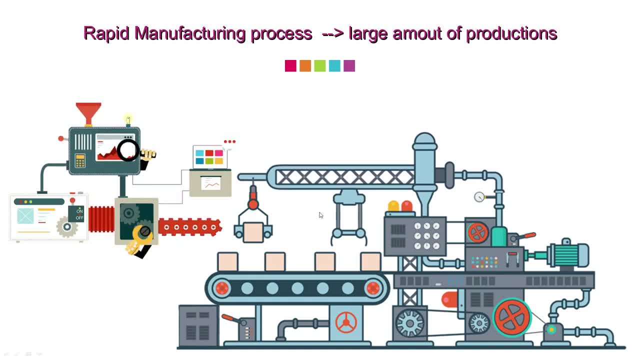 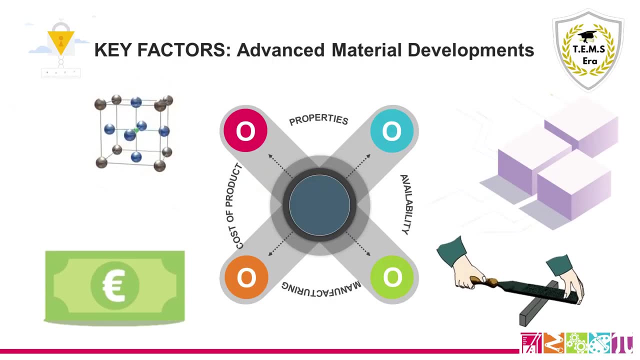 productions will be available and obviously easy manufacturing should be there for rapid manufacturing process so we can achieve a low cost. now, moving to the very next uh thing was a cost of the product. now, of course, the purchase cost may be a material cost we talk, or if we talk about. 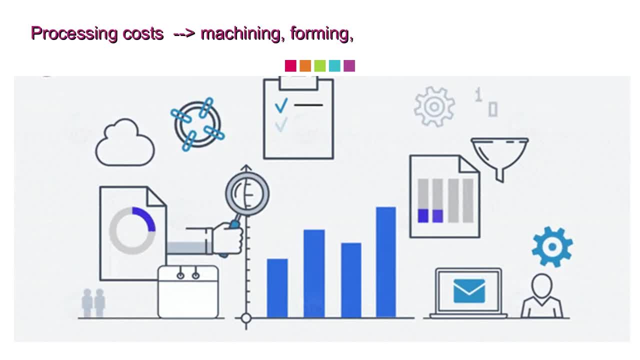 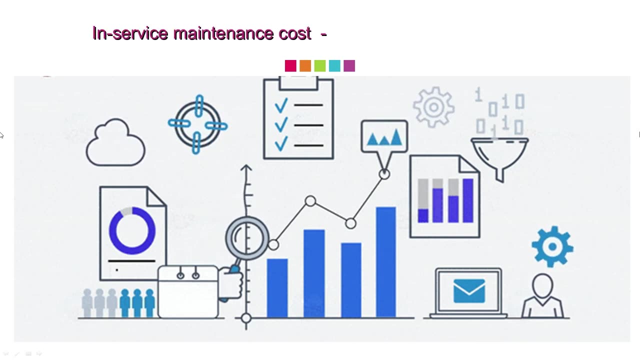 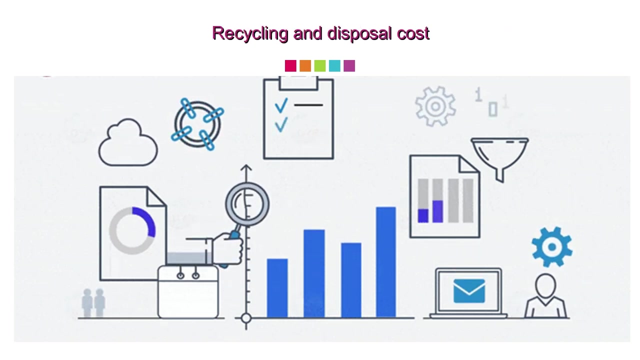 the cost of the aircraft. yes, the purchase cost must be reduced. then processing cost must be taken care properly. that includes machining, forming, shaping or even heat treatment cost. uh, also in service maintenance cost, which also includes inspection or the repair cost. and of course you must think about recycling and the disposal cost. so you might have seen a spacex line. 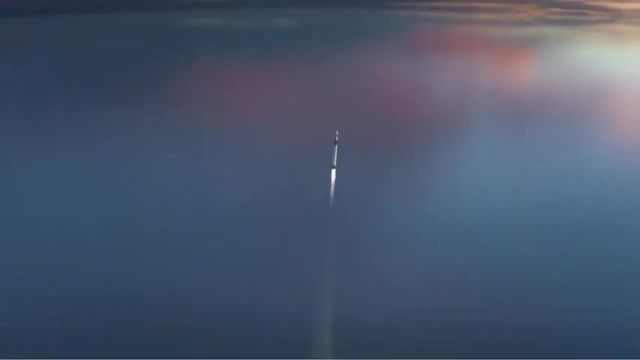 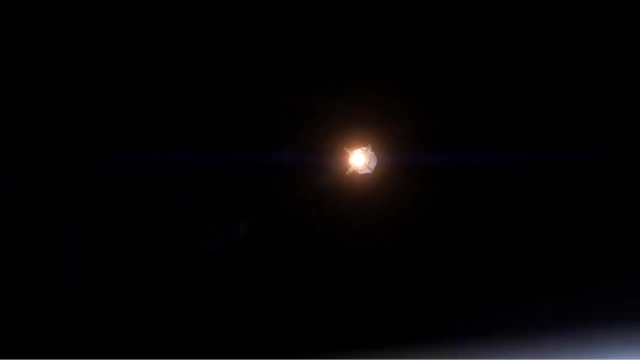 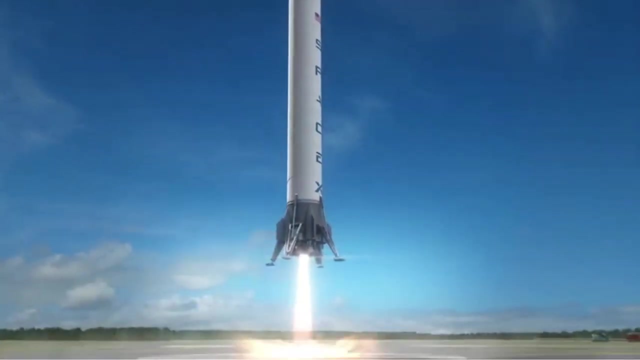 launch. they have used reusable launch vehicle. due to use of that launch vehicle, they can decrease or cut off the huge amount of overall cost of this project. so you can understand how this cost, directly or indirectly, play a greater role in that. here comes, uh, the table which gives. 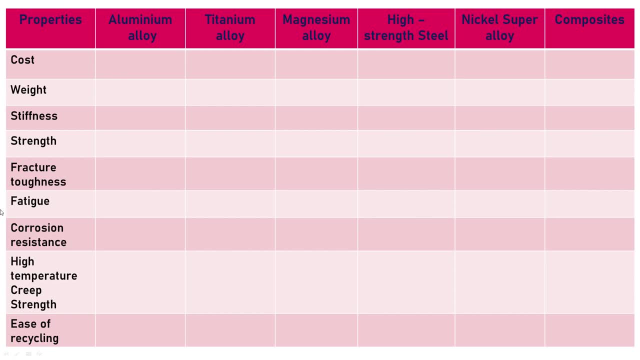 approximate grading of an common aerospace material for an several key factors and the properties for an airframes and the engines. so here are the key uh properties, as you can see: cost, weight, stiffness, strength, fracture toughness, fatigue, corrosion resistance, high temperature, creep strength. and the easy or ease of reciting, and we have the several well commonly. 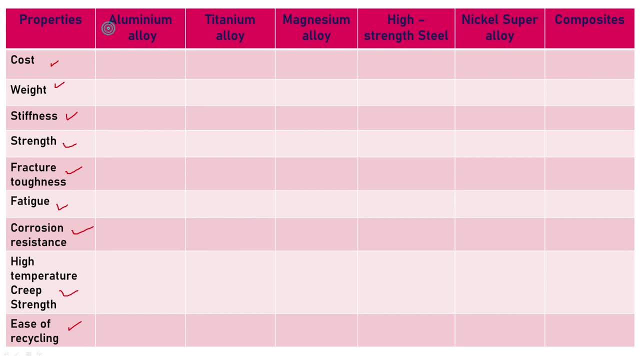 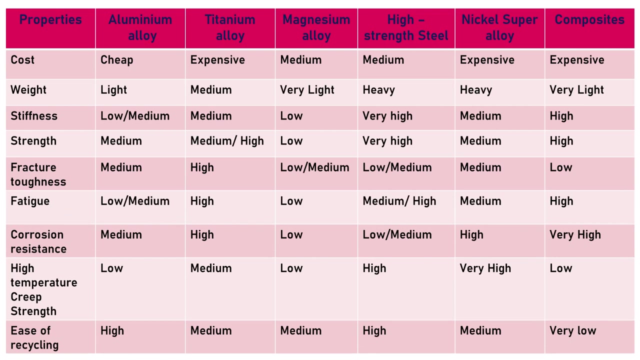 known type of materials, such as aluminum alloy, titanium alloy, magnesium alloy, high strength steel alloy, nickel, super alloys and, of course, a composite composite material. so these are the well-known uh materials and now you can see the gradings has been done based on the properties and the material, which one is cheap and which one is expensive? uh, which one is lightweight, which is? 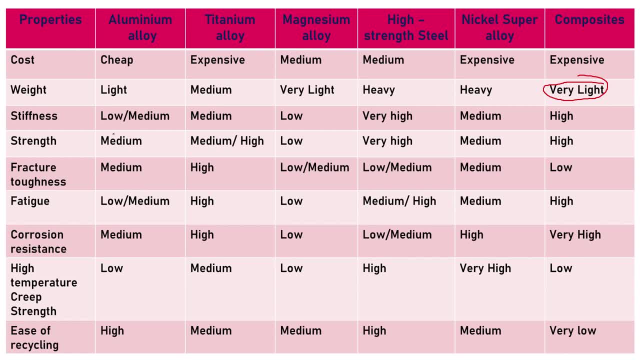 very lightweight. so which one you need to compromise, which one will be. you need to uh, based on this chart, based on your requirement, you need to optimize your data, uh, and you have to find out again these four parameters, how you're going to optimize based on these four parameters, and you have to um, bring that to in some conclusion, and not only that. 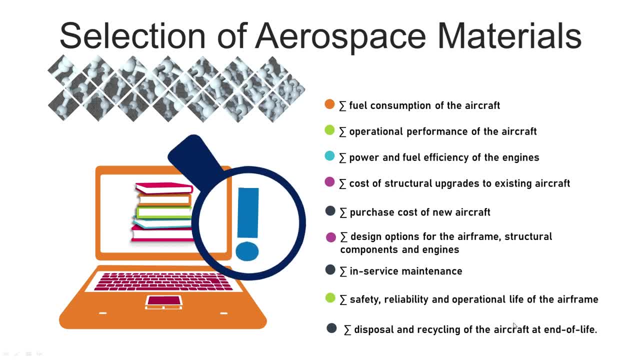 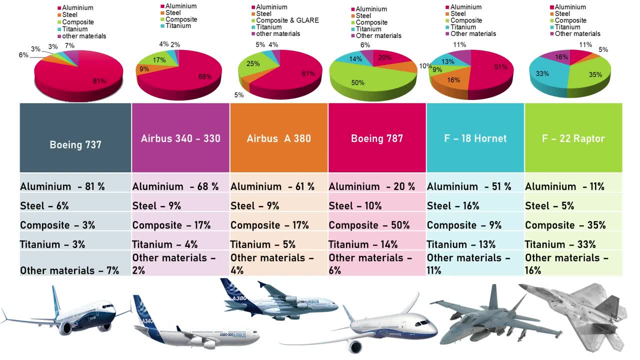 this will give you a better idea once you have the literature review or little survey for your particular aircraft. here i've done a literature survey for boeing 737, airbus 340, 330 and 737, airbus a380, boeing 787 and also some of the military aircrafts like f-18, hornet and f-22. 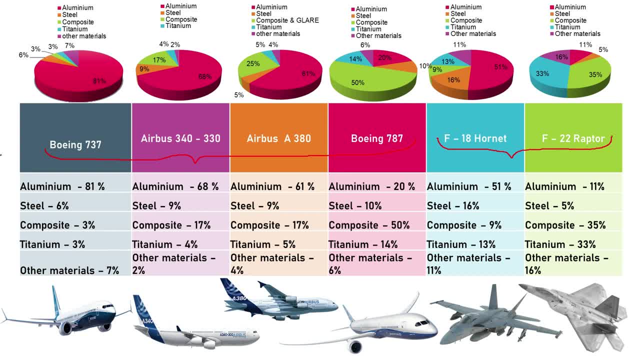 raptor. so based on that you can see the compositions or the majorly used materials in that particular aircraft. you can see for a passenger aircraft which is can say only this month, like boeing 737 to boeing 787, that the drastically the use of aluminum has been. 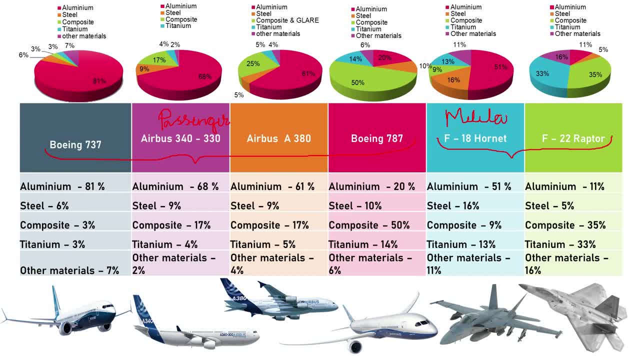 increased and, if you see, the usage of composite has drastically increased. so, uh, this, these are the overall uh percentile, or you can say the major of that. you know the majority of the materials used in the aircraft. now, second step: what you have to do is uh that the more details need to be studied. that is here the major materials used in the aircraft. 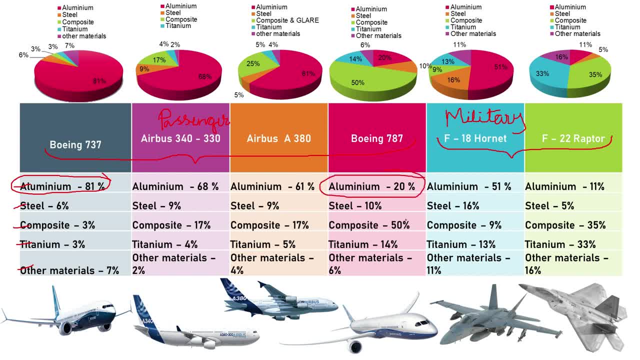 suppose if i talk about aluminum, if i talk about, you know that high strength steel, composite titanium and any other extra materials. so more details, you must need to study to understand which. if i talk about aluminum, which aluminum alloys are used that you want to understand and that 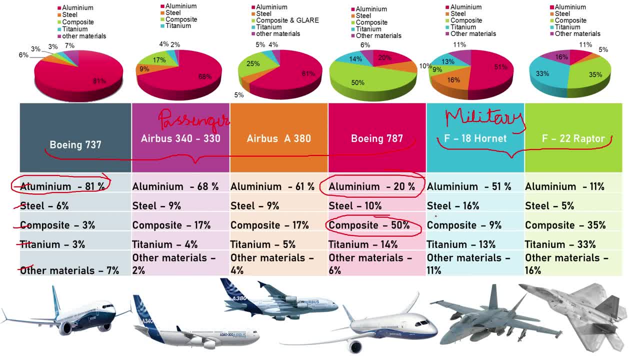 aluminum alloys where it is located, like where it is used. it is used in the wing or the fuselage, or they have used that uh aluminum, that much percentage of aluminum, because in the later part of this uh program you also need to find out or predict for an you know. 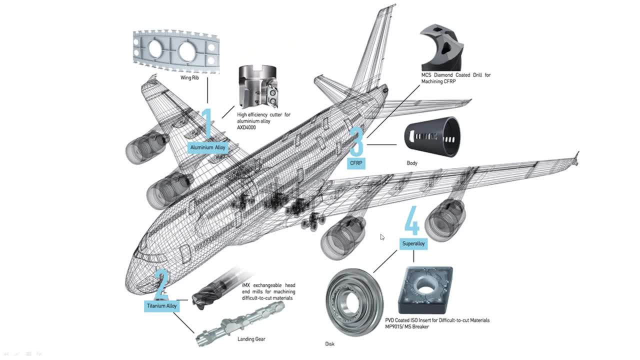 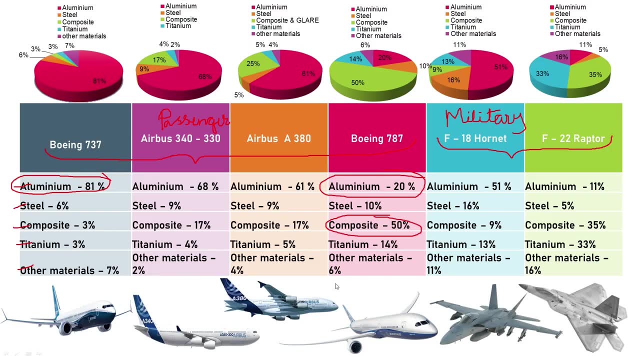 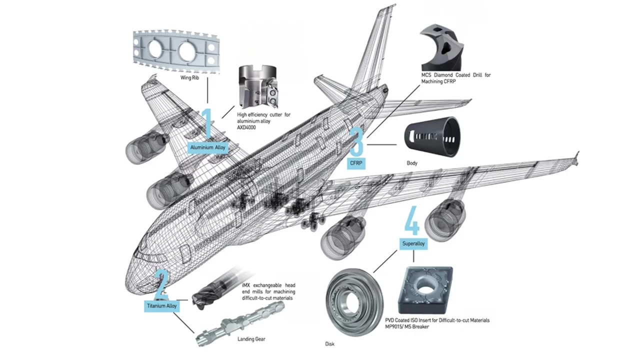 for an individual weight. and the individual weight of a seat- uh. individual center of gravity of an individual component. so in that regards you need to find out the weight of individual component. if i talk about wing, fuselage, landing gear, engine- uh, horizontal tail, vertical tail- all you need to find out separately and the material used in it. so here also we will talk. 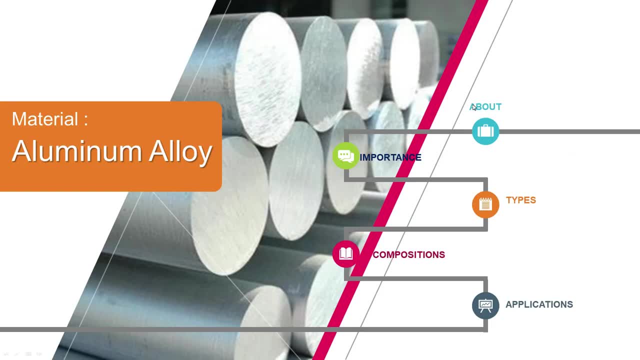 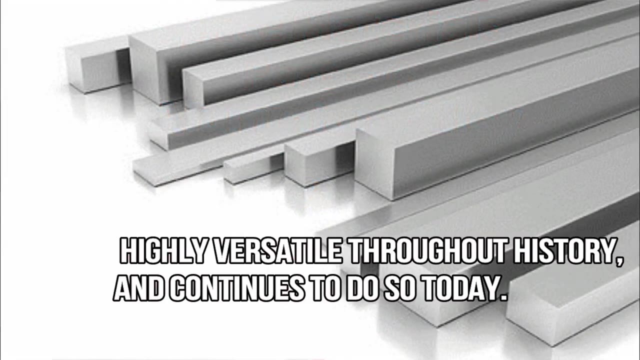 more about the composite material. so before that, uh, starting one by one. the first starts with aluminum. aluminum is a material of choice for most aircraft structures and it has been started since 1920s to early 50s. Aluminum has proven highly versatile throughout history and continuously to do so today. 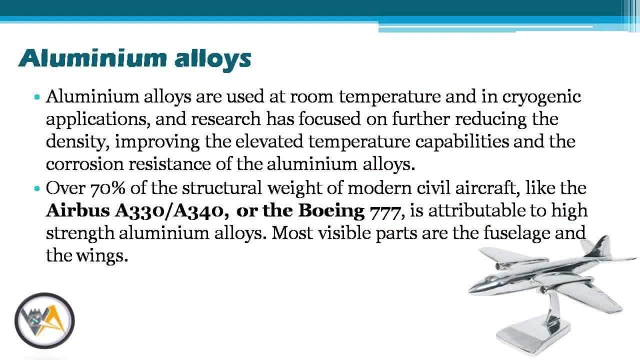 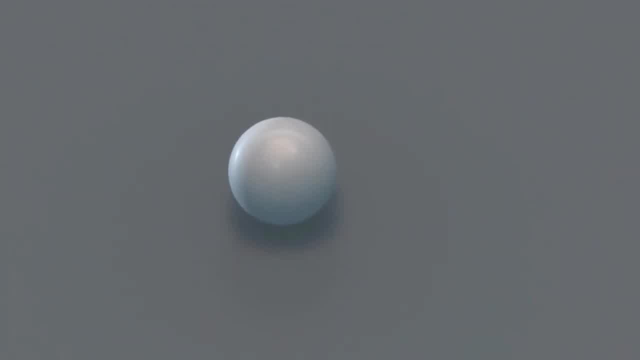 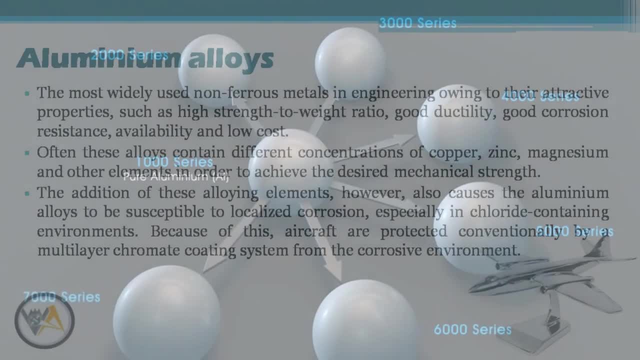 aluminium alloys are basically used at room temperature and in electronic applications, and research has focused on further reducing the density and improving the elevated temperature capability and the corrosion resistance of the aluminum alloys. Aluminum alloys are most widely used non-fiber alloy. Aluminum alloy is used in most of the year, although it is not good for the 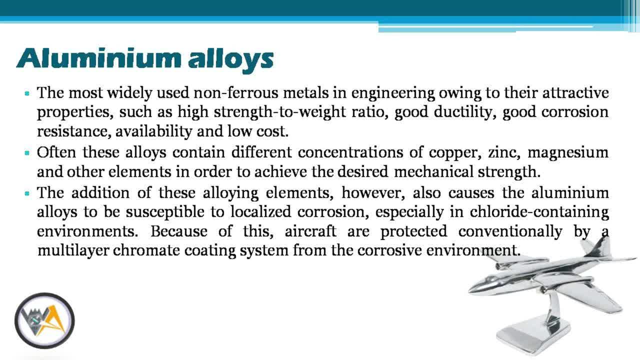 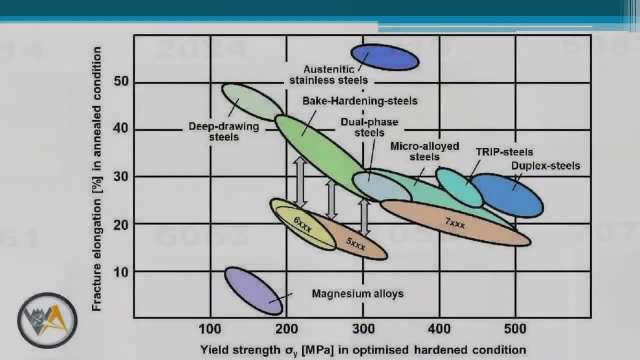 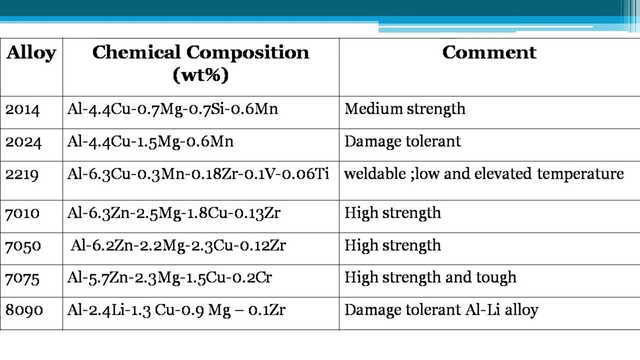 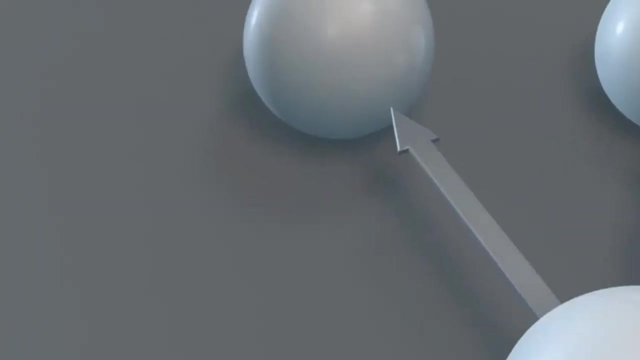 ferrous material in engineering owing to an attractive properties such as high strength to weight ratio, good ductability, good corrosion resistance, availability and low cost. there are a number of different types of aluminium alloys, but are some suitable to the aerospace industries than others. example of such aluminium includes 2024, the primary alloy element in 2024 aluminium. 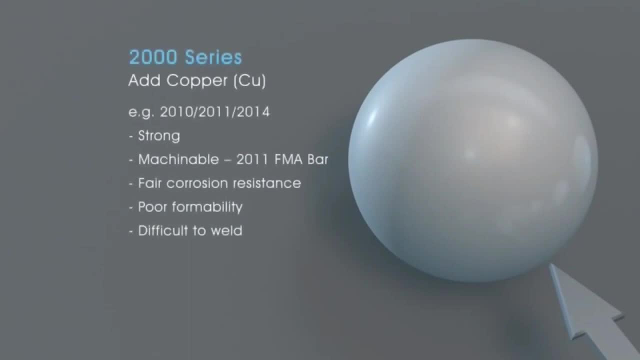 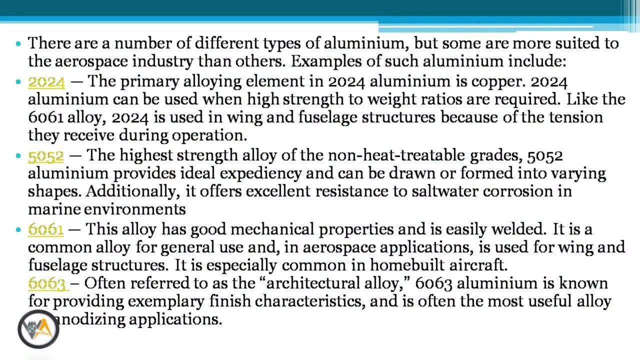 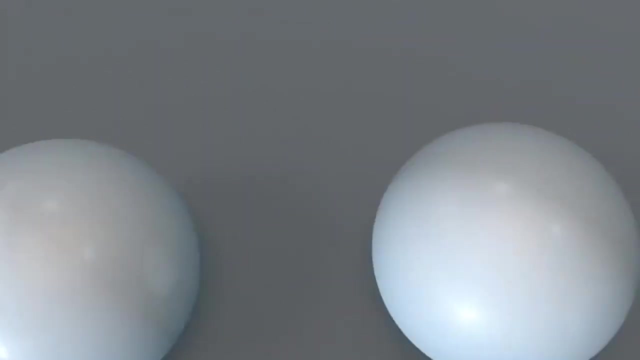 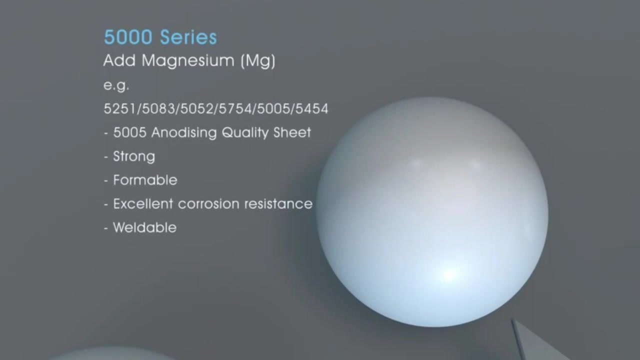 is copper. 2024 aluminium can be used when high strength to wear ratios are required. 2024 is used in wing and fuselage structure because tension they receive during operation. 5052, the highest strength alloy of the non-heat treatable grade. 5052 aluminium provides ideal expandancy and can draw or form into various shapes accordingly. 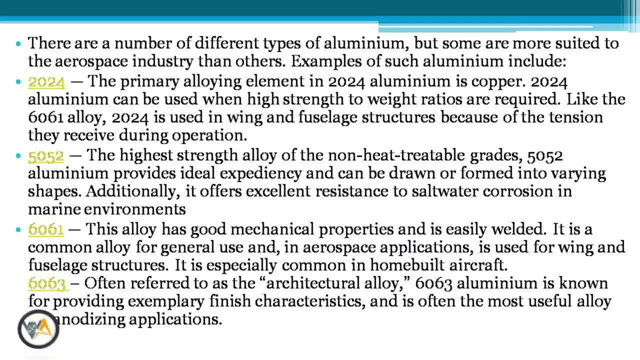 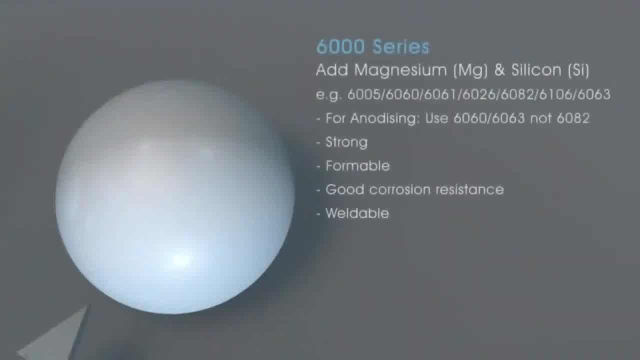 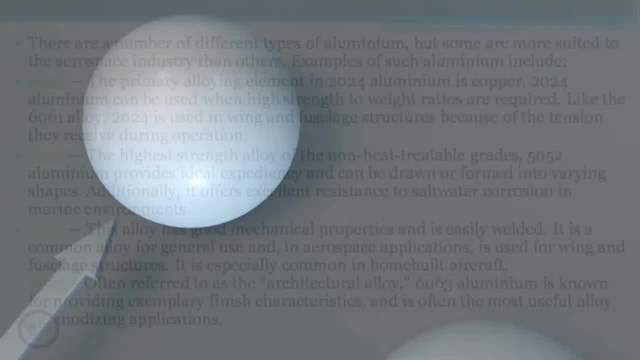 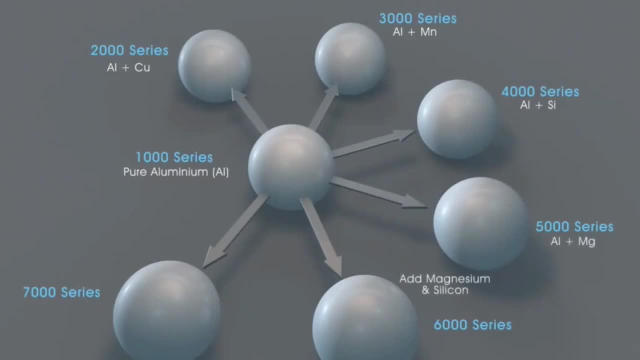 in addition, it offers excellent resistance to salt water corrosion in marine environments. 6061: this alloy has a good mechanical properties and it's easily welded. it's a common alloy for general use and in aerospace applications. 6062: it is used for wing and fuselage structure. it's it is especially common in home-built aircraft. 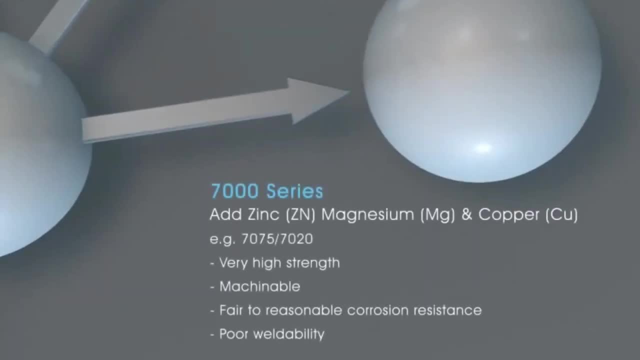 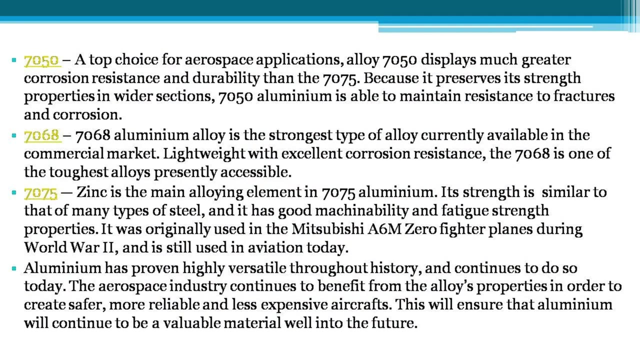 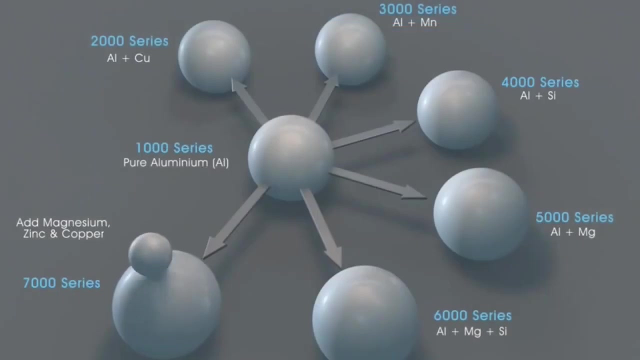 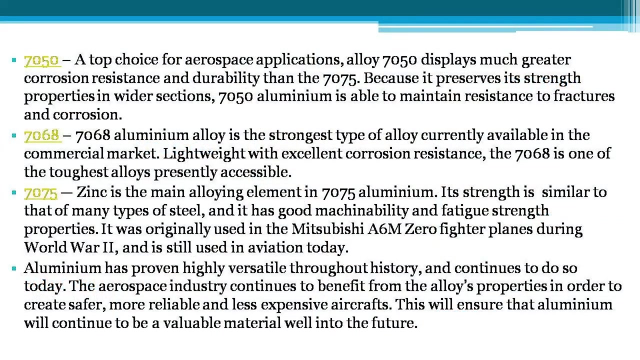 7050, a top choice for aerospace application. alloy 7050 displays much greater corrosion resistance and durability than 7075 because it prevents its strength properties in widened section. 7050 aluminium is able to maintain resistance to fracture and corrosion. 7068 aluminium is the strongest type of the alum alloy currently. 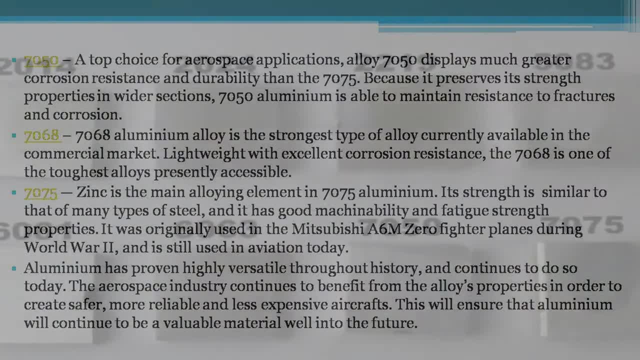 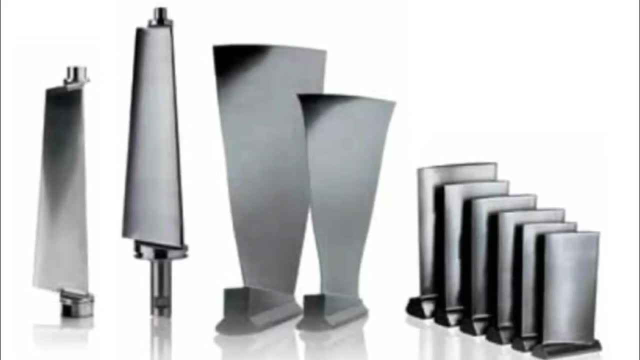 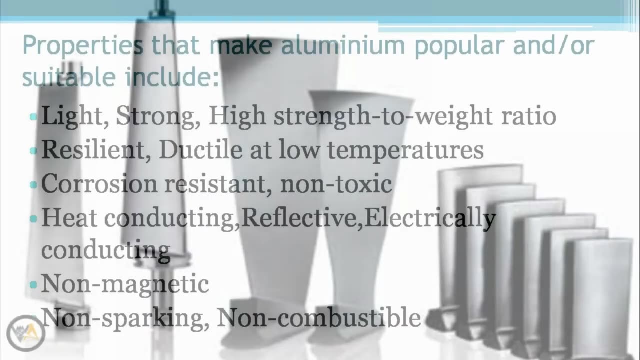 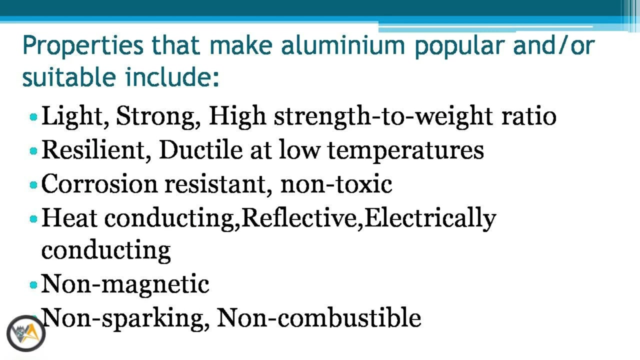 available in the commercial market. lightweight and excellent corrosion resistance. the 7068 is one of the toughest alloy presently accessible. aluminium in the engineering material of choice for many applications. properties that make the aluminium popular and suitable includes: light, strong, high strength to bed ratio, resilient, ductile at low temperatures. 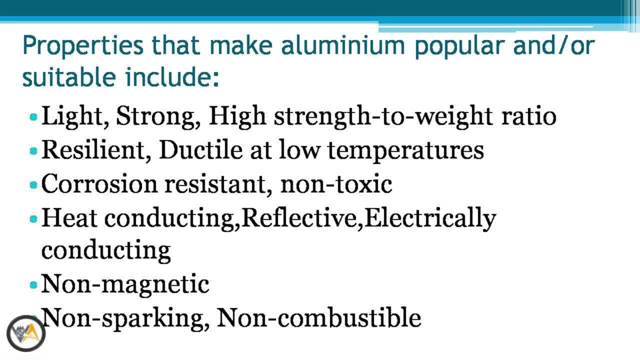 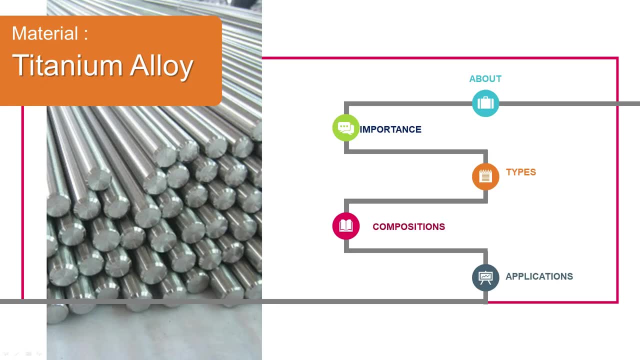 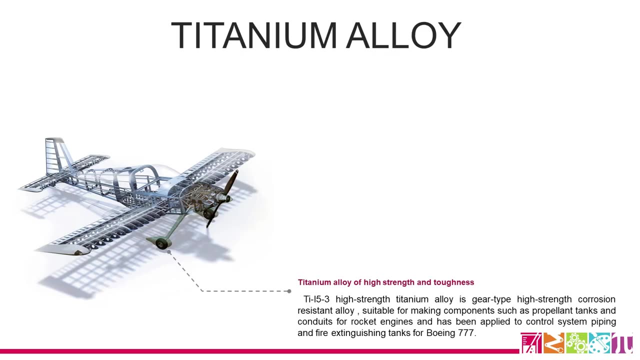 corrosion resistant, non-toxic heat conducting, reflective conducting, electrically conducting, non-magnetic, non-sparkling and non-combustible. so titanium alloys are used in both the air frame structures and as well as a jet engine components because of their moderate weight and high structural properties. now, if i talk about high structural properties means stiffness, strength. 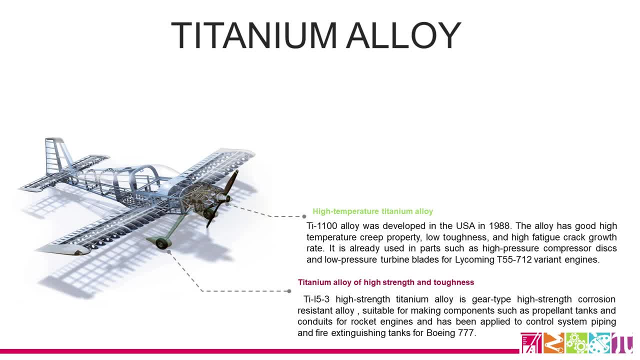 toughness and fatigue. and also they must have the excellent corrosion resistance and the ability to retain their property- mechanical properties- at a very high temperature. so this is a key quality for a titanium alloys. 7083- a top choice for aerospace application. 7063 am a top choice for emergency use and 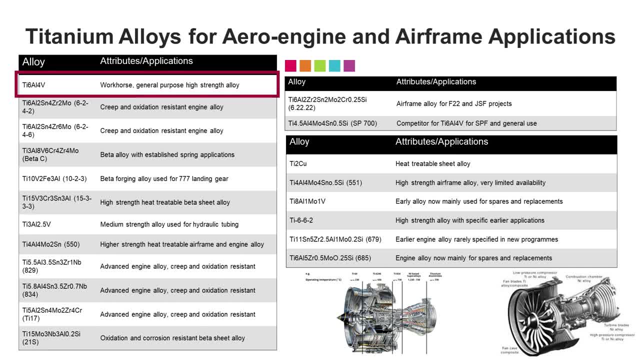 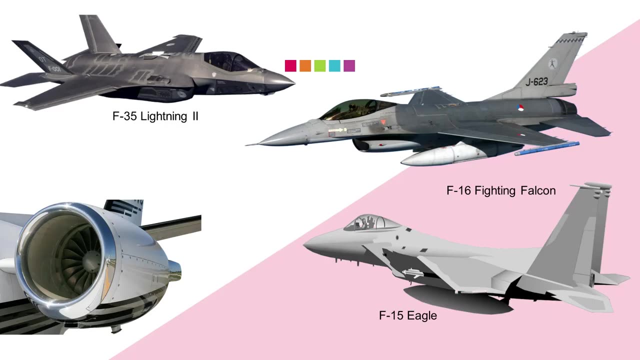 Apart from that, there are so many varieties of titanium alloys, with different compositions, which are used, So, although the most common type is Ti6Al4V, that is, titanium, 6-aluminium and 4-valadium So, which is used in both the aerospace or the aircraft structures and the engines. 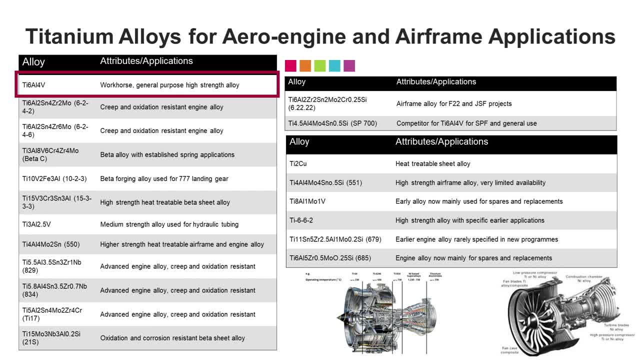 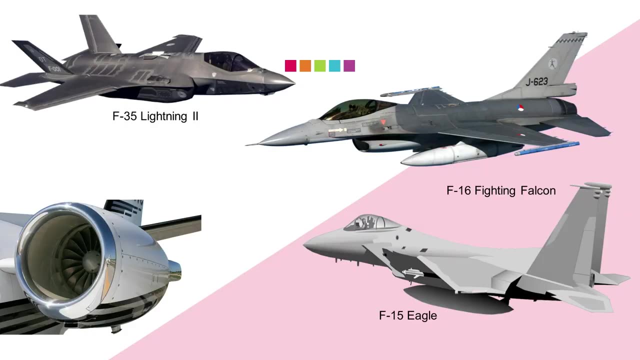 The structural properties of titanium are better than the aluminum, although it is more expensive and heavy. Titanium is generally used in the most heavily loaded structures that must occupy minimum space, such as landing gear and wing fuselage connections. The use of titanium is greater in fighter aircrafts owing to their needs. 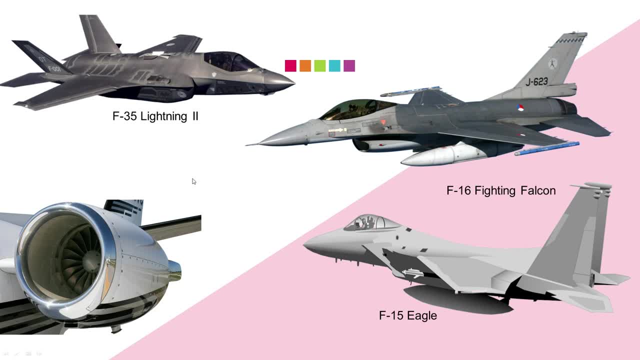 So, apart from that, if you look in the case studies like, titanium accounts about 25% of the structural mass of an F-15 Eagle, as well as F-16 Fighting Falcon, and 35% of the structural mass of F-35 Lightning II. 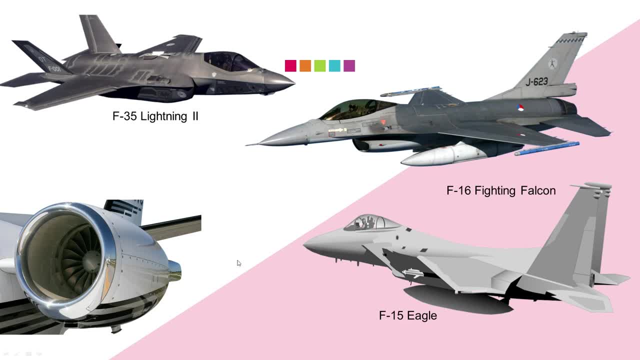 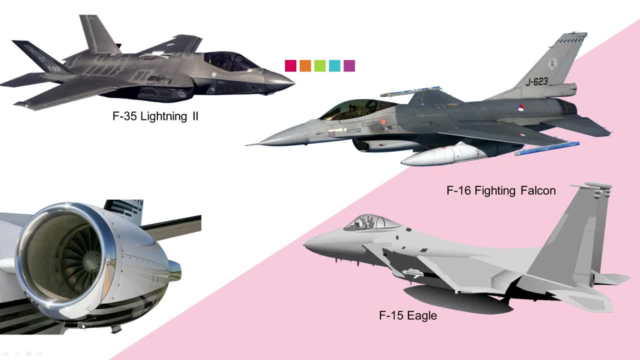 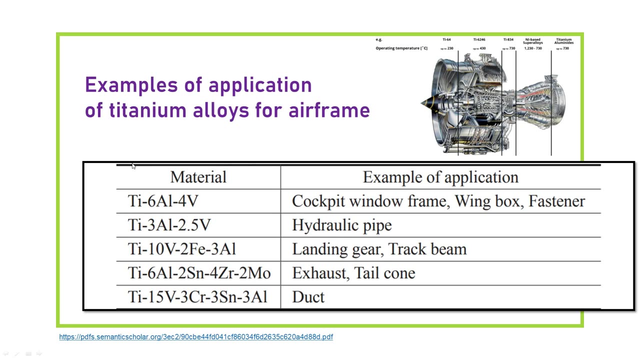 are used in the components required to operate under 400-500-degree centigrade And in the engine components made up of turbine titanium, including fan blades, low pressure compressor parts and plugs and nozzle assemblies in the exhaust chamber, or they can say exhaust session section. so this is all about this titanium, so more when you want to. 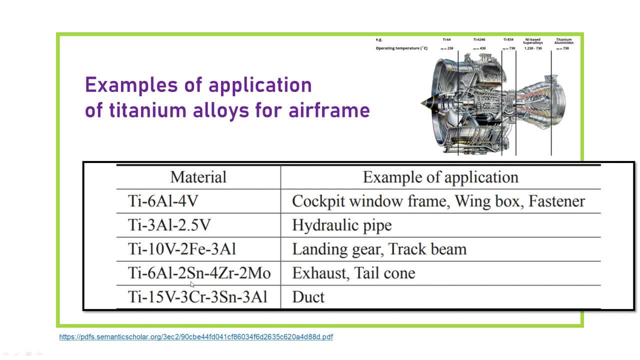 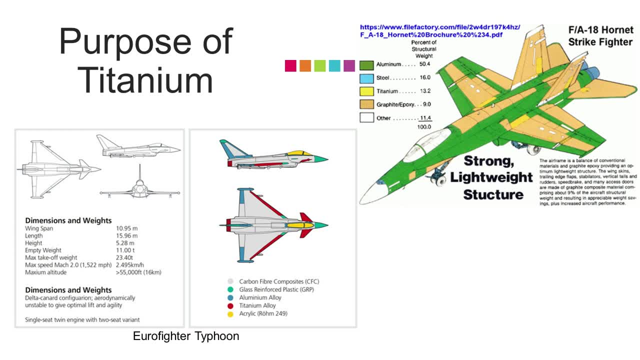 study about the each and every applications of particular aircraft. so in deep you have to study, so in major, uh, the outline of the titanium application is: it save weight, having it resist a resistance of heat, resistance to embrittlement at low temperature, high corrosion resistance and the low thermal expansion. so these are the key points about this titanium alloy. 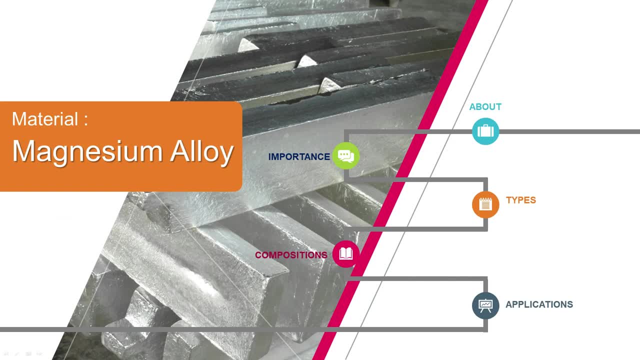 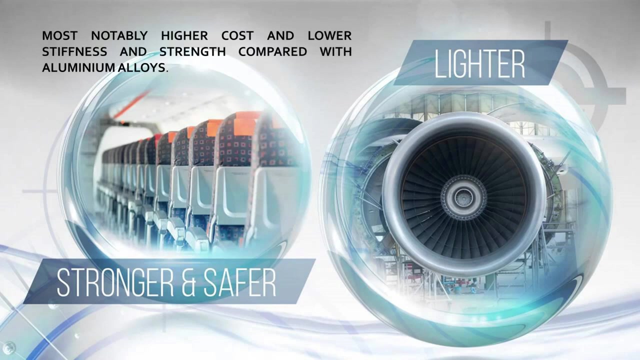 and now talking about magnesium. the magnesium alloys is one of the lightest materials and for this reason was a most popular material for the lightweight aircraft structures, and this magnesium was been extensively used in aircraft building during 1940s and 1950s. the main reason to reduce the weight: 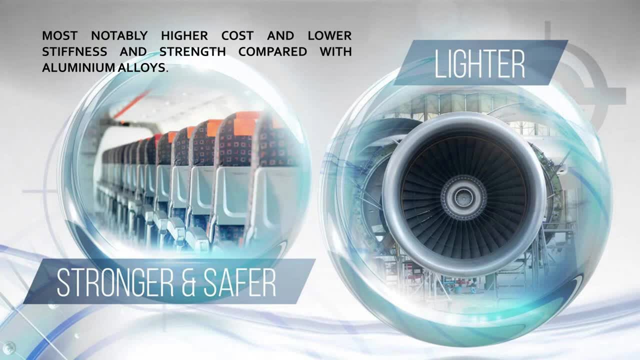 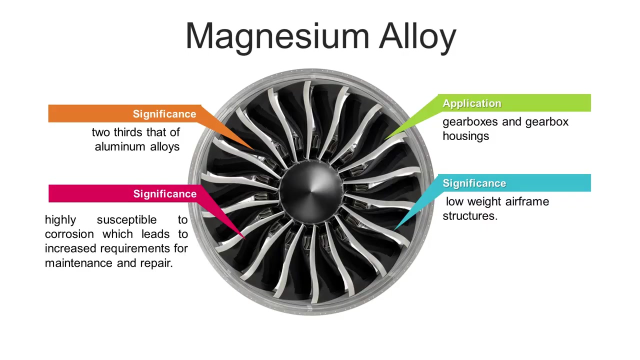 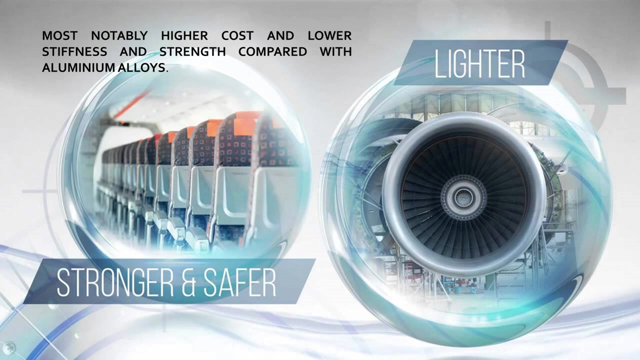 but since there was some usage has declined as it has been replaced by aluminium alloys and composite. now the use of magnesium in the modern aircraft and the helicopters is typically less than of total structural weight. now diminishing of magnesium as an important structural material has been caused by several factors. the most notably is the higher cost. 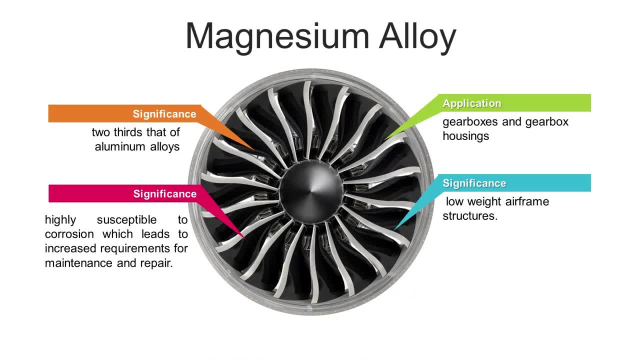 and low stiffness. strength compared with aluminium alloys is quite low, so magnesium is highly susceptible to corrosions, which lead to an increase in requirements for maintenance as well as further repair. the use of alum magnesium alloys is now largely confined to non-gas turbine engine parts, and application includes gearbox or an gearbox housings of. 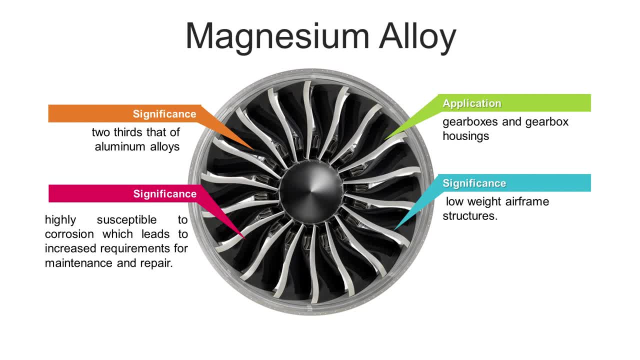 piston engine aircraft and some of the main transmissions housing of helicopters. so we don't use much of it. but the magnesium alloys have also been attractive to design due to their low density- uh, only two-thirds of the density, or two-thirds that of the aluminium alloy in the aerospace industry- and therefore can be an innovation technology if used for a low weight. 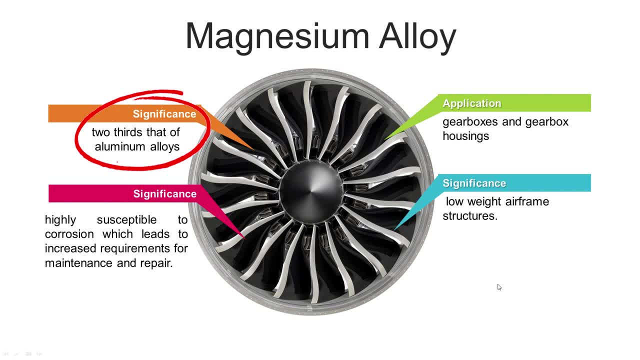 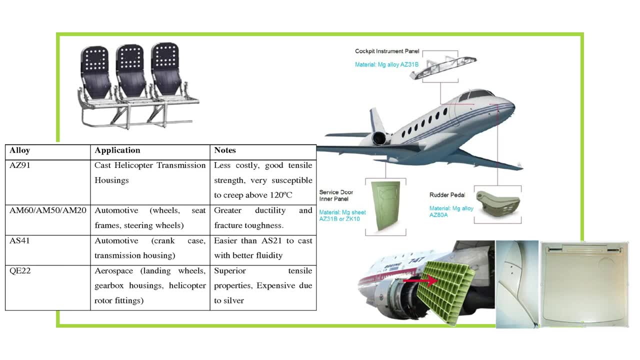 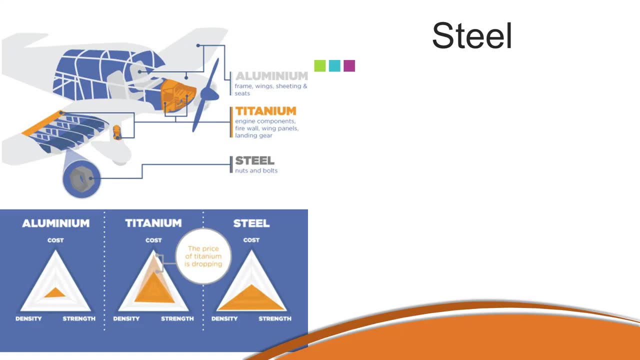 airframe structures and this has been major factor in the wide spread of magnesium alloy casting and the and its products. okay, now talking about this high strength steel, steel is mostly used in the production of aluminium alloys. the steel used in aluminium alloys is mostly or commonly used metal in a structural engineering. 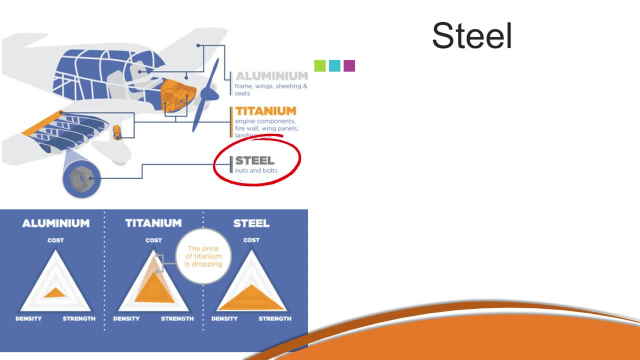 however, it is used as a structural material in an aircraft is small, under five to ten percentage by weight. now, the steel used in the aircraft are the alloys or the heat treated for an high, very high strength and about three times stronger than the aluminium and twice as strong as titanium. 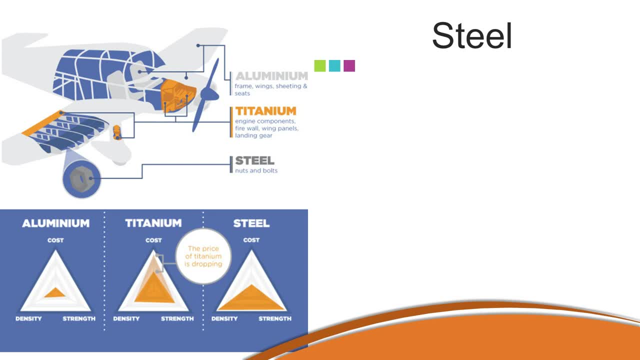 steel has a very high young's modulus, or you can say three times stiffer than the aluminium. so together with an good fatigue resistance and as well as the fracture toughness, so steel is also extensively used in engine and exhaust components. so mostly used for the corrosion resistance and 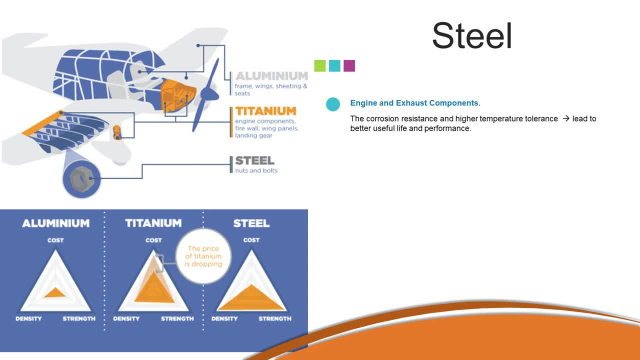 the high temperature tolerance of an stainless steel, so aerospace component, which can lead to and performance. now talking about landing gear, yes, it is used because it causes a high uh tensile, uh strength and shear modulus. often, stainless steel makes it more suitable for absorbing the impact stress during landing and uh and helps to given better endure. so okay, so one more: is that key uh? 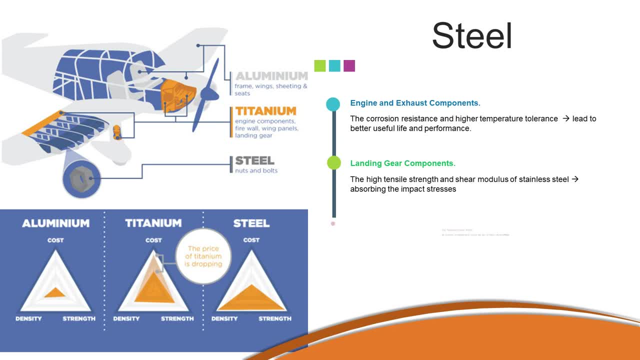 superstructure joints. so this aerospace stainless steel can be used to for enough key joints in an aircraft superstructures to improve the durability and reduce the risk of failure during flight. and so these are the few factors, key factors about the steel and then, last, i will talk about the composite material. space explosions has come. 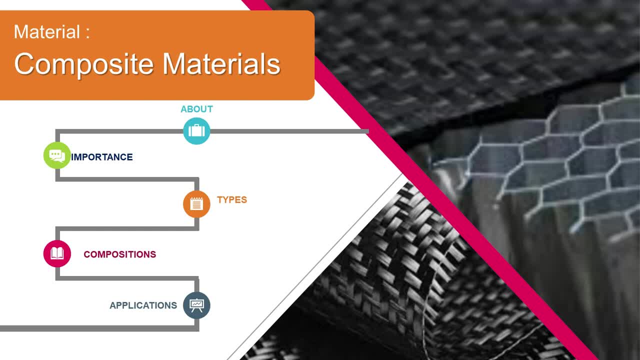 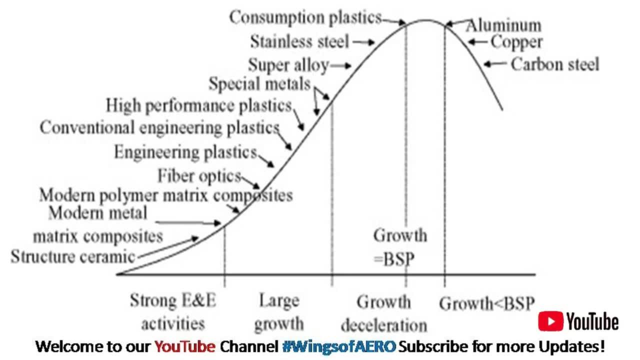 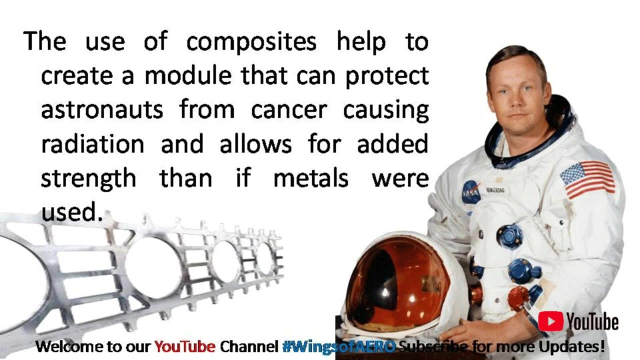 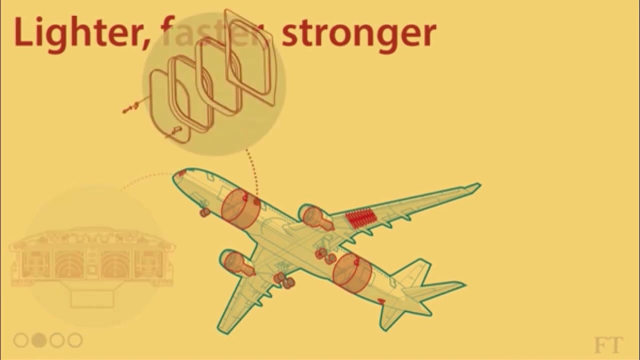 a long way since neil armstrong first walked on the moon in 1969.. the use of components helped to create a module that can protect astronauts from cancer causing radiation and allows for added strength than it if the metals were used. additionally, composite can be refined. 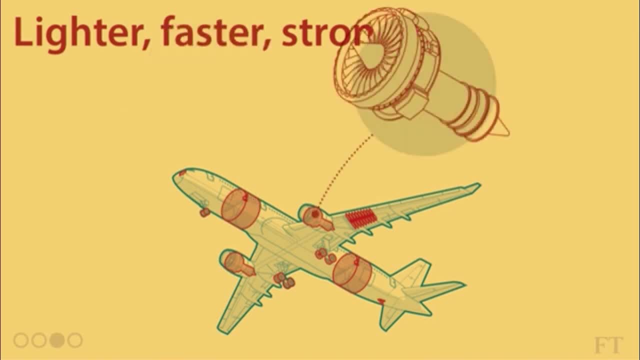 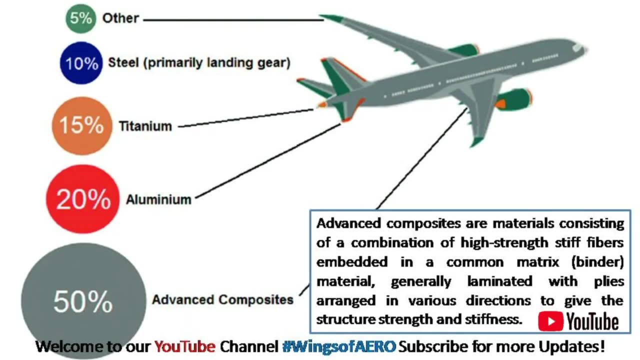 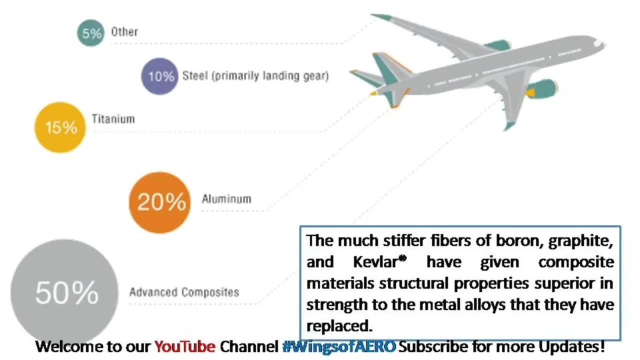 where is y tested, are constantly performed in the quest for stronger and lighter materials. advanced composites are materials: materials consisting of a combination of high-strength, stiff fibers embedded into a common matrix, material generally laminated with piles arranged in various directions to give the strength of the structure and the stiffness. 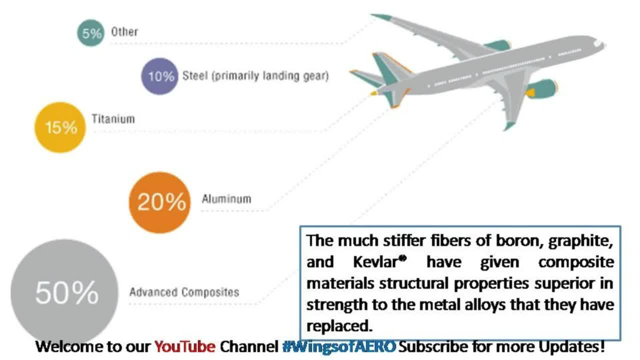 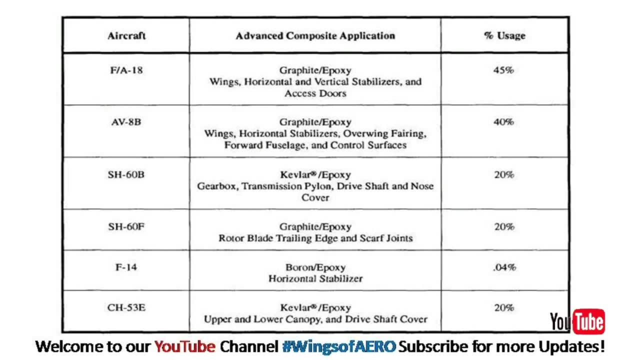 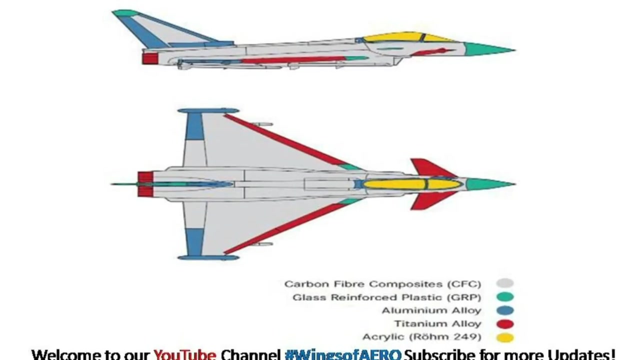 The much stiffer the fibers of boron, graphite and kevlar have given the composite material structural properties superior in strength to the metal alloys that they have replaced. Specific applications of advanced composite materials. an approximate percentage of the total aircraft structures for some of our modern-days aircraft are shown in your screen. 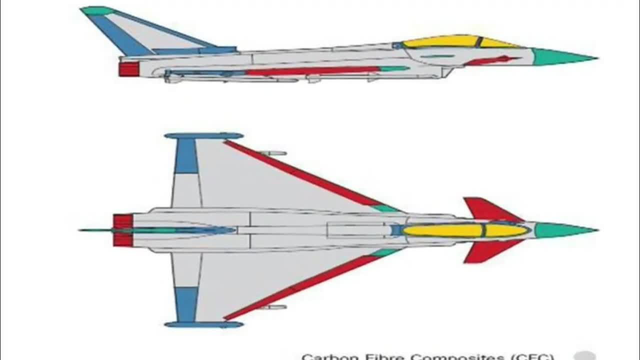 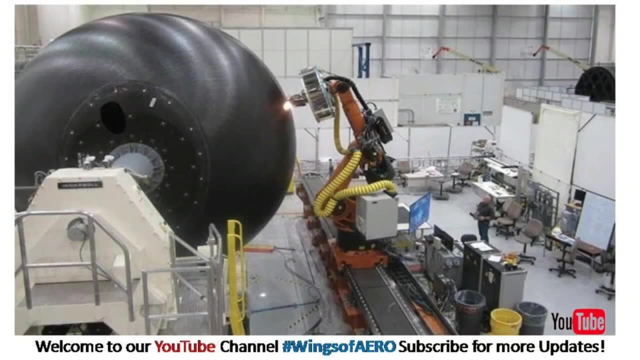 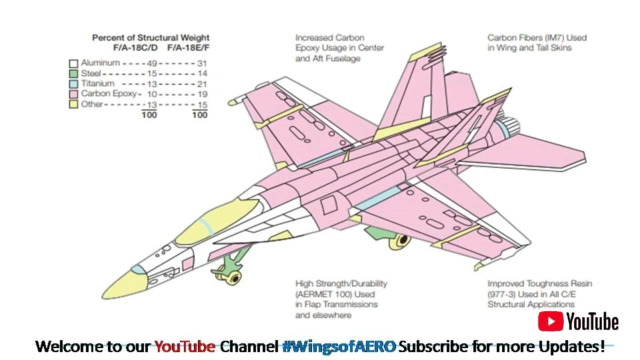 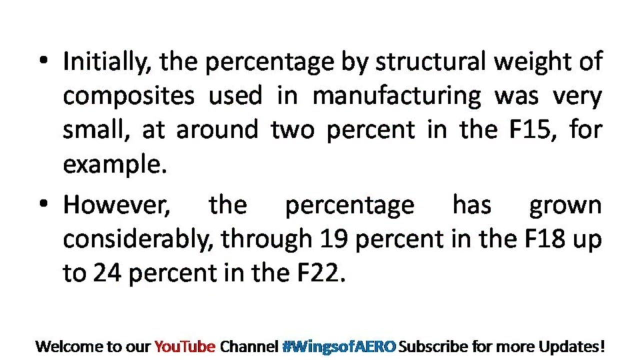 Among the first users of the modern composite material was about 40 years ago when boron-reinforced epoxy composites were used for the skin of an amphibious of US F-14 and F-15 fighter aircrafts. Initially, the percentage by the structural weight of the composites used in manufacturing. 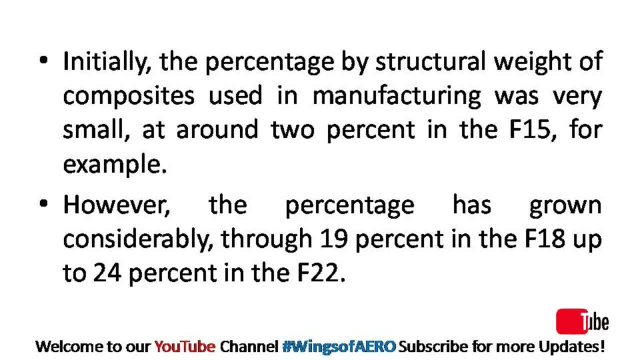 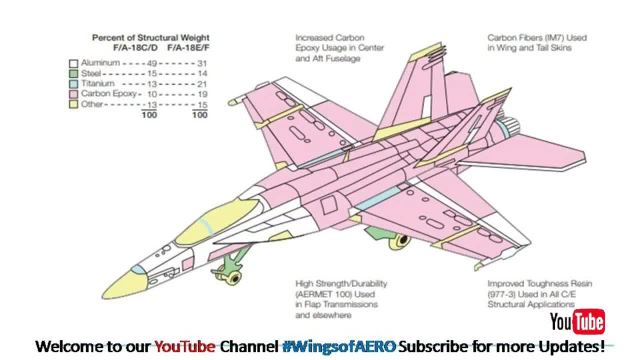 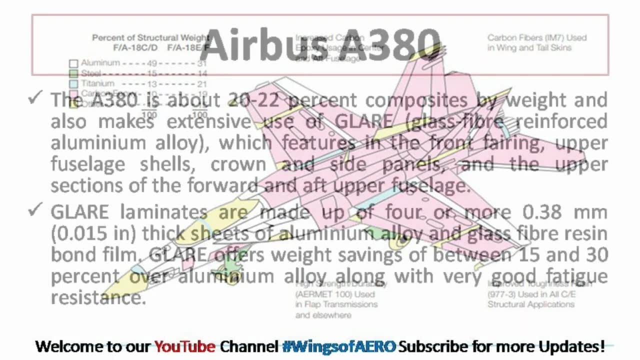 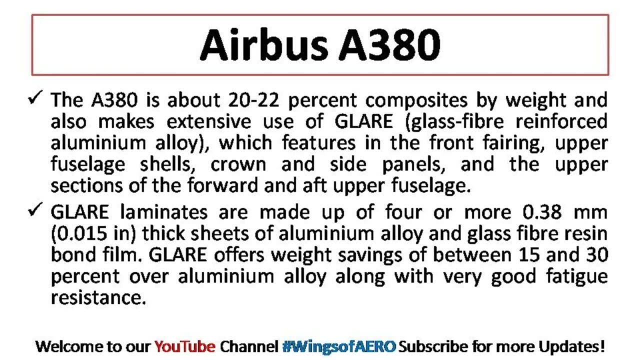 was very small, at around 2% in F-15, for example. However, the percentage has increased. The percentage has grown considerably throughout 19% in F-18, up to 24% in F-22.. Airbus A380 is about 20-20% of composites by weight and also makes extensive use of. 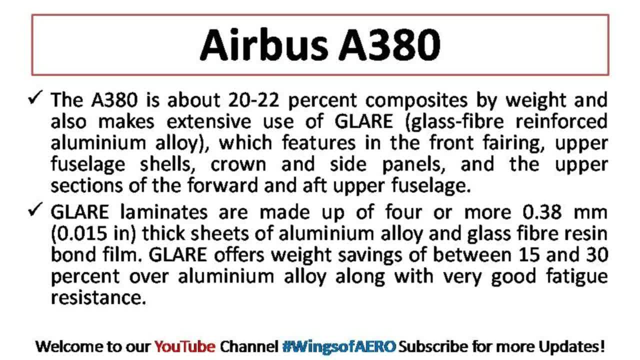 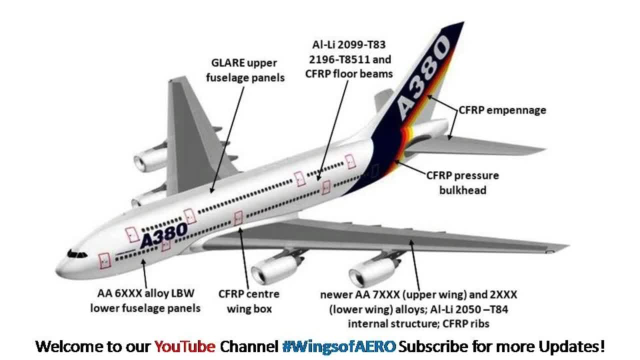 glass fiber reinforced aluminum alloy which features in front fairing, upper fuselage and cell and upper sections of the forward and after upper fuselage. 2. Glass Fiber Reinforced Aluminum Alloy Laminates are made up of 4 or more 0.38-meter. 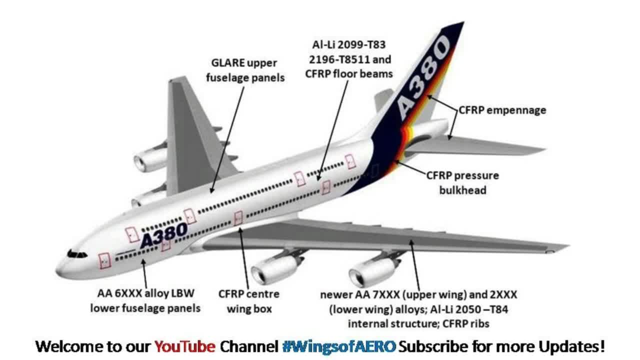 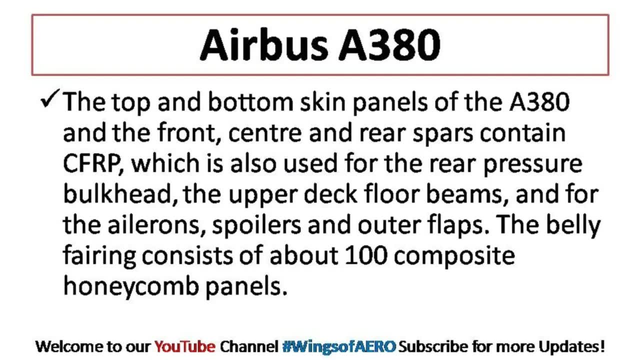 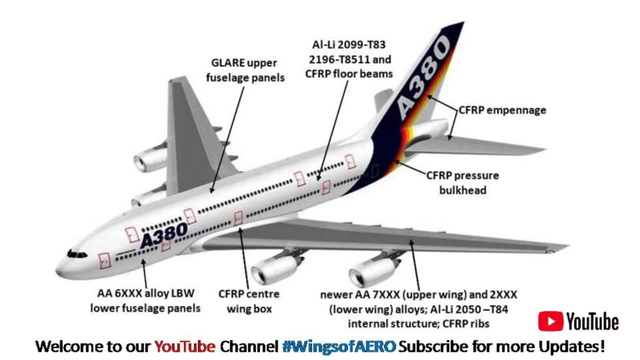 thick sheets of aluminum alloy and the glass fiber resin bond film. The top and the bottom skin panels of Airbus A380 and the front center panel of the 3.5-inch A380 are made out of accurately visible aluminum. 2. center and the rear spark containing CFRP, which is used in the rear pressure bulkhead. 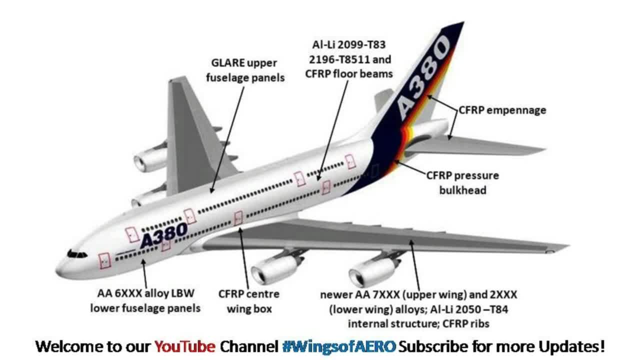 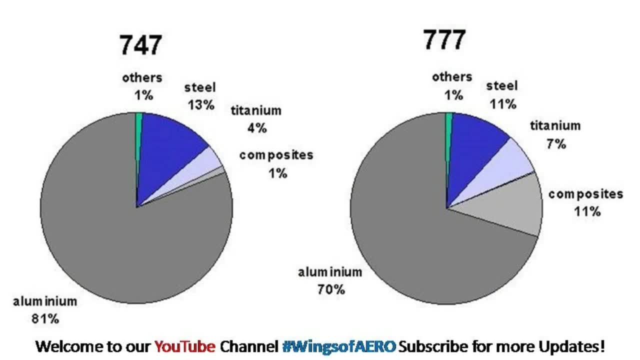 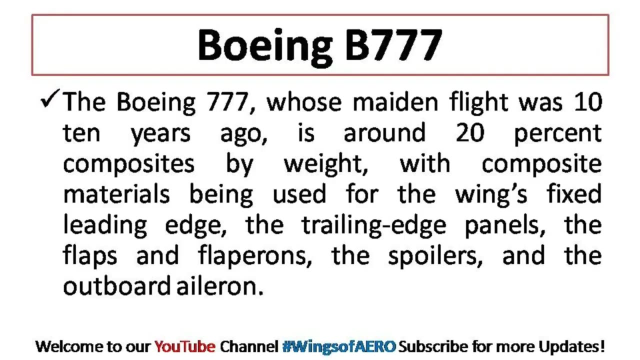 and the upper deck floor beam and for the aileron spoiler and the outer flaps. Boeing 777,, whose main flight was 10 years ago, is around 20% composites by weight, which, with composite materials being used for the wing's fixed leading edge, trailing edge panel. 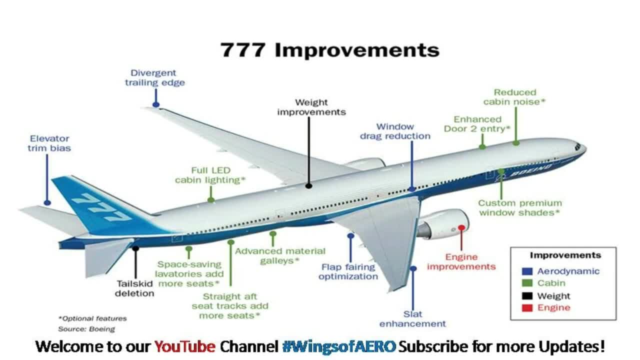 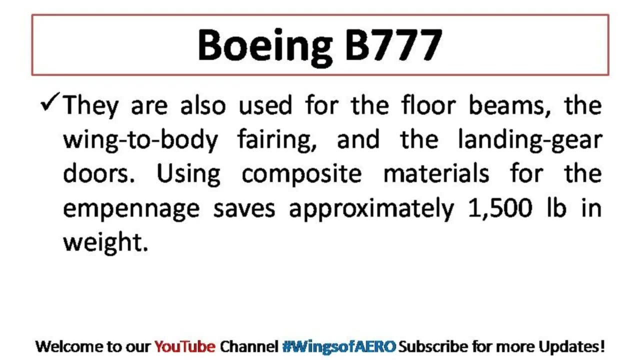 flaps, flap-arounds, spoilers and the outboard aileron. They are also used in the floor beams, wing-to-body fairings, landing gear doors. Using composite material for the amphenages saves approximately 1,500 pounds in weight. 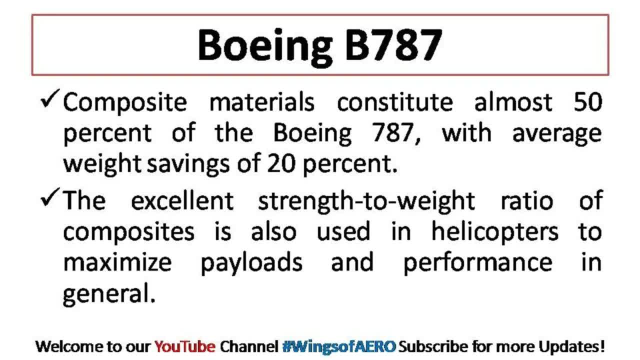 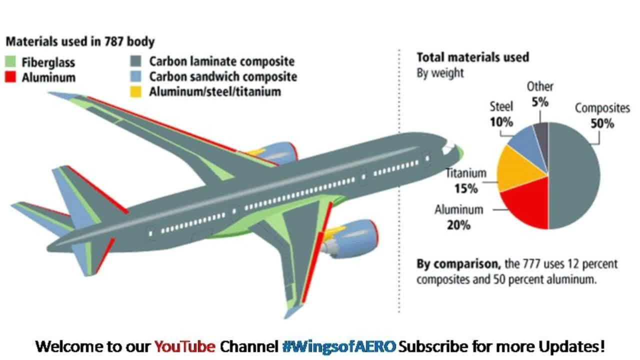 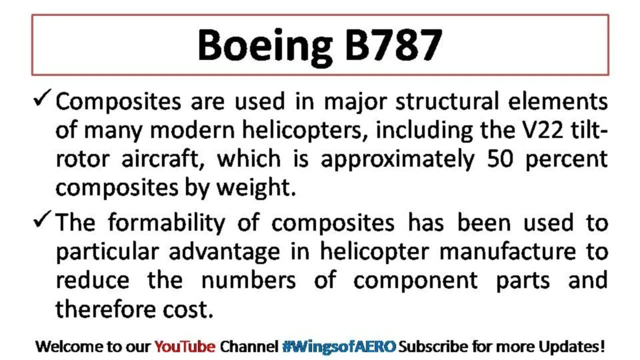 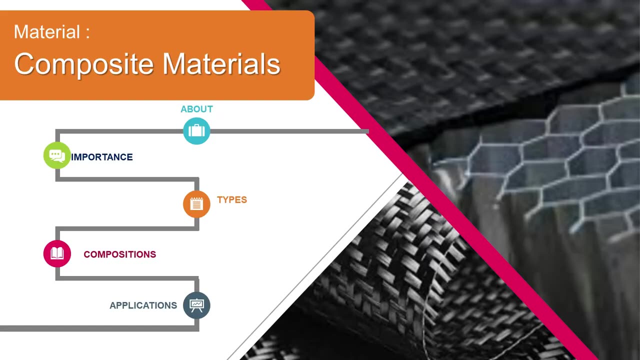 Composite material constitutes almost 50% of the Boeing 787, with an average weight saves of 20%. The excellence, the strength-to-weight ratio of composite is also used in helicopters to maximize the payload and performance in general. So you know what is composite material. yes, it is a combination of one or more materials. 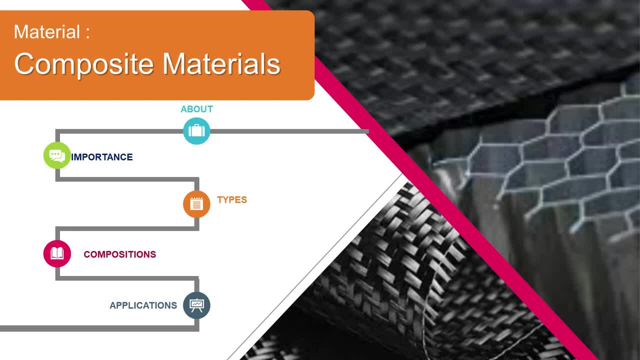 compiled together. And what is composite material? Composite material is a composite material that is made up of a set of materials and both are having some significant different physical or maybe of chemical properties, And when they mix together and bind it together, and it gives separate or distinct features. 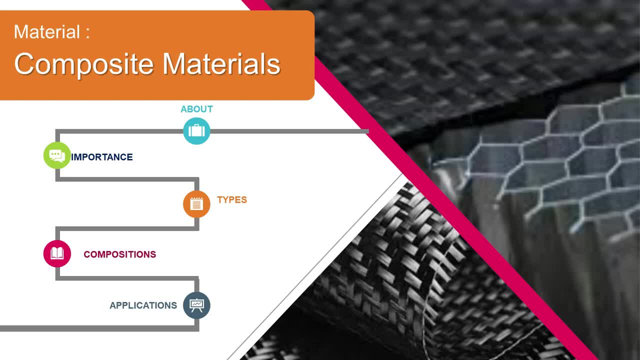 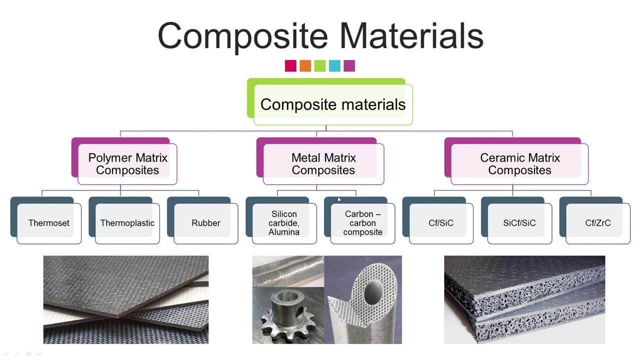 or separate material properties. So this is all about composite material and it can be classified in three types. First one is a polymer matrix composite. Second is a metal matrix composite And the third one is a ceramic composite. So there are so many types, each types having their own applications. 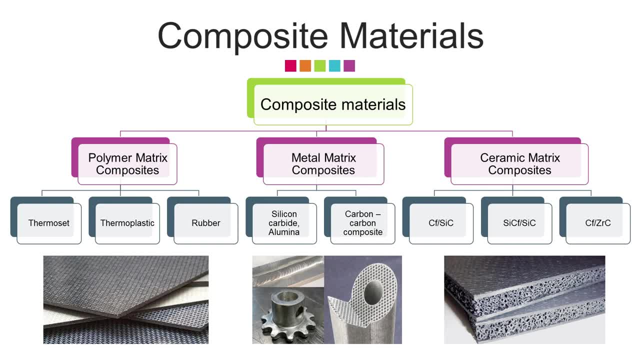 So, based on that particular thing, having so many types of varieties of resin, that most common was a polystyrene, vinyl, or there is epoxy, is there? So these are the very common types And similarly, you might be knowing about the common fibers, that is, glass fiber, carbon. 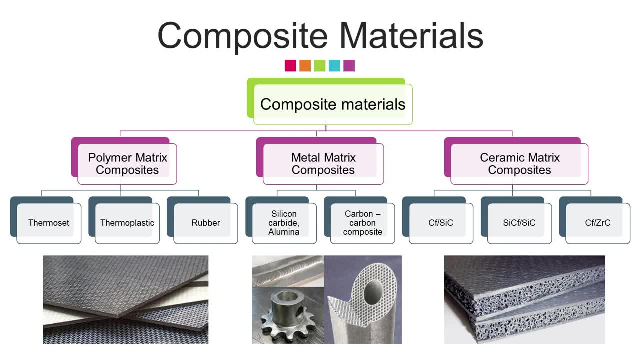 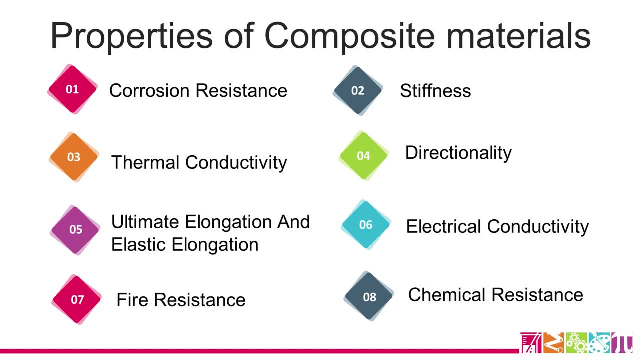 fiber, I'm read, boron all those things. The properties of a composite are greatly influenced by the orientation and the nature of those fibers. So we won't see much of that composite material because it is complete, a very huge, huge. 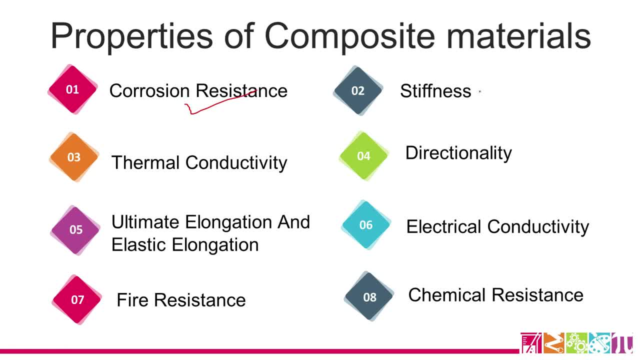 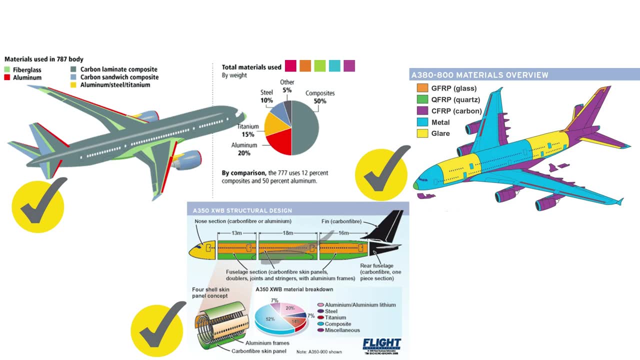 huge scope for, or a huge platform to, learn more about the composite. So if you want to know more about the composite, I will drop a link over in the somewhere in the description On the top of the description, so you can find more lectures about the composite from. 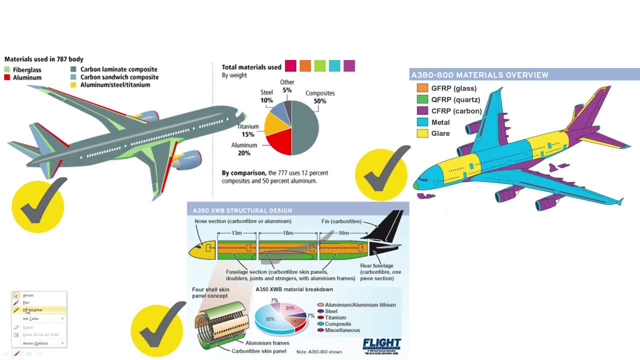 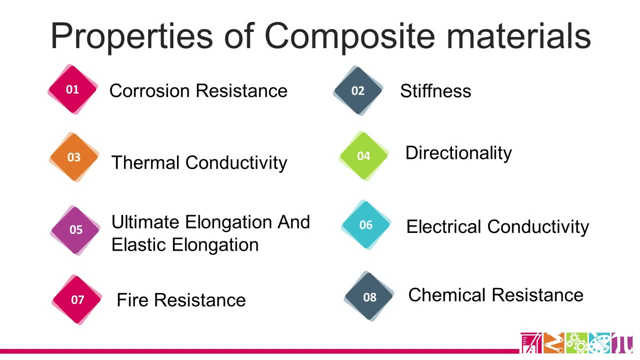 IIT Jammu. So yes, so coming back to that, how to? here we are talking about how to select a material in our aircraft, So before that you must know a few properties about this composite material. So here you need to understand the properties of the polymer composites. 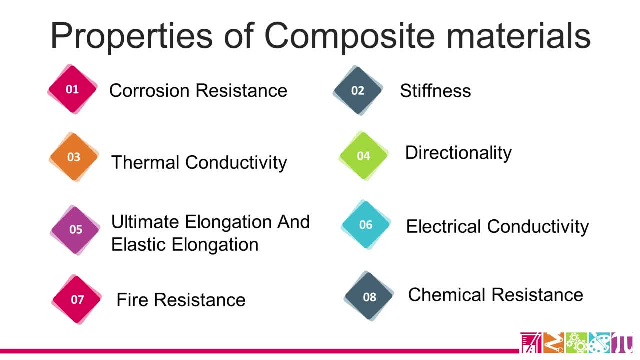 So, accordingly, the composite materials you can select On your aircraft to aircraft. So those are the properties like corrosion resistance, stiffness, high conductivity, directionality, then ultimate elongations and elastic elongations. Not only that, electric conductions, replaceability for materials, heat stabilizers, fire resistance. 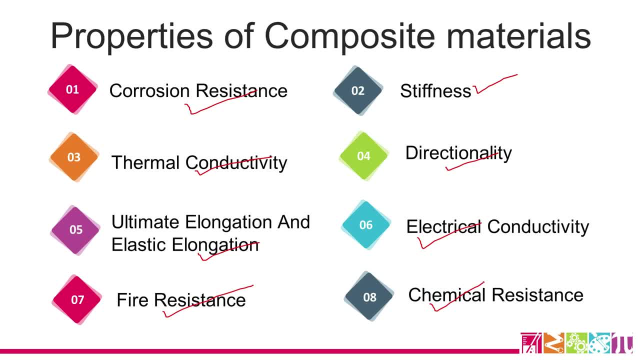 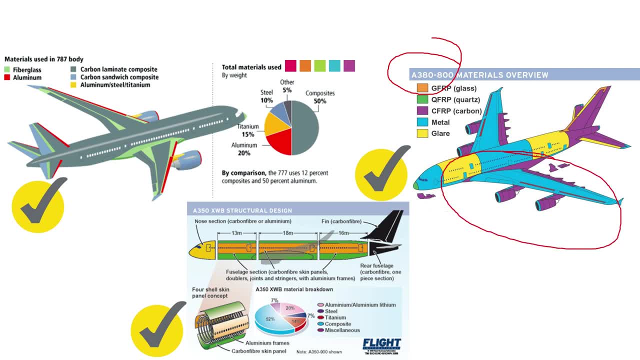 fire resistance, chemical resistance and property based on performance benefits are following. So many people have a few of them, Okay, So let's start with the questions like: why are the composite material using aircraft right Now? composite material are important in aviation industry because they provide a structural 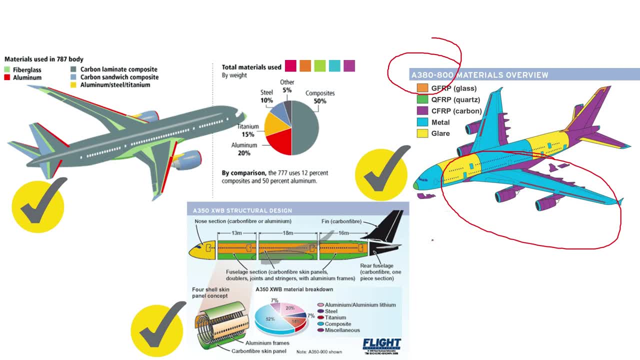 strength compared to metallic alloys and, in addition, to a lighter weight. So this leads to an improve in fuel efficiency and which is directly connected with the performance of an aircraft. So that's the main reason why the composite material is widely used. Okay, Now the question is what composites are mainly used in the aircraft. 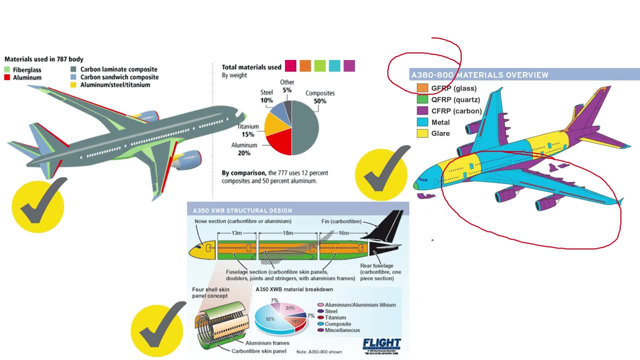 Yes, the, as I've said, the composite material have played a major role in weight reduction and today there are of three types already I've said so. among that, the most classic and the most rapidly used one are the carbon fiber, glass fiber aramide, reinforced epoxy. 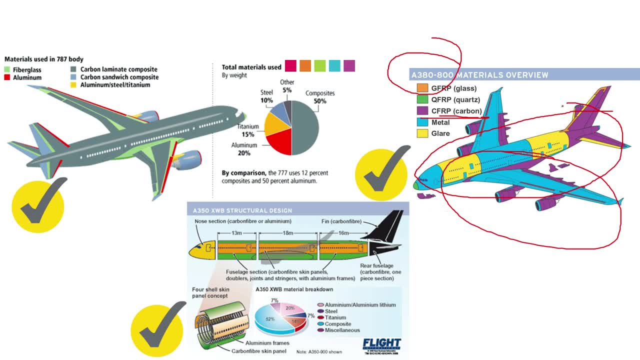 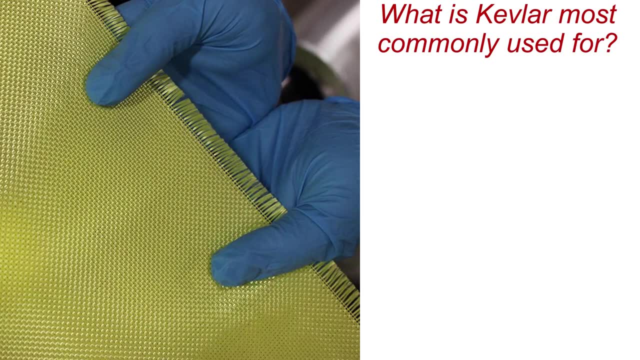 Kevlar. There are other composite materials like wood. There are other composite materials like wood. There are other composite materials like boron, reinforced composite material and so on, And Kevlar is one of the most common composite material that is used. 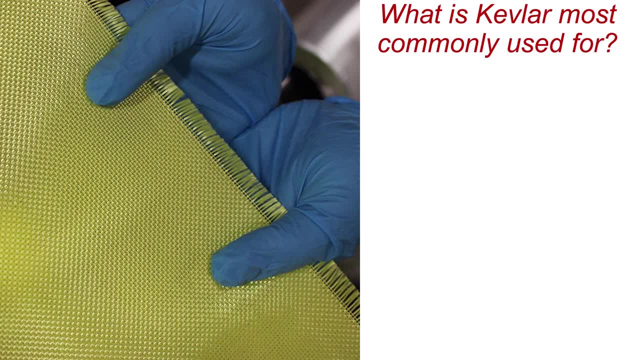 The reason is the Kevlar fibers helps to deliver a durability, lightweight, stiffness and thermal as well as fire protections in an aircraft components, And this Kevlar gives an remarkable performance in increasing the fuel efficiency, decreasing the operating and the manufacturing cost. 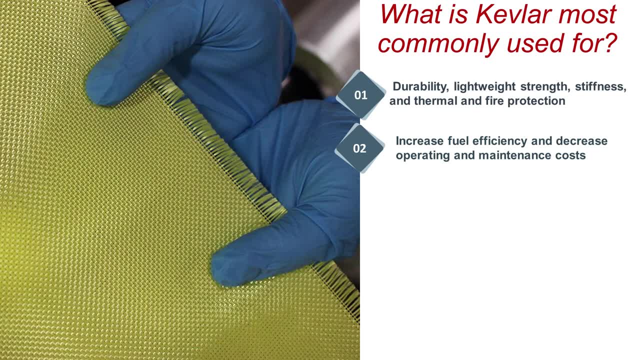 So this Kevlar plays a very unique property of a high strength, high toughness and the chemical stability at a very high temperature. This Kevlar are mostly widely used in the friction materials. Mostly, you can see, you know, combustion protection materials in an aerospace and other components. 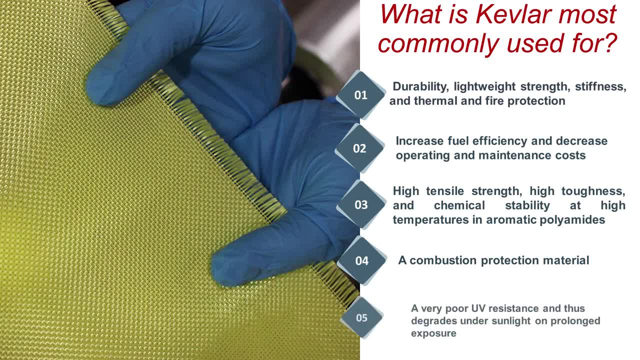 of an aircraft, But it also having some disadvantages. The main disadvantages are that it is having a very poor UAV resistance, right? So yes, one more of the most frequently asked question now, what type of Kevlar it is. Mostly it is used Kevlar 29 and Kevlar 49.. 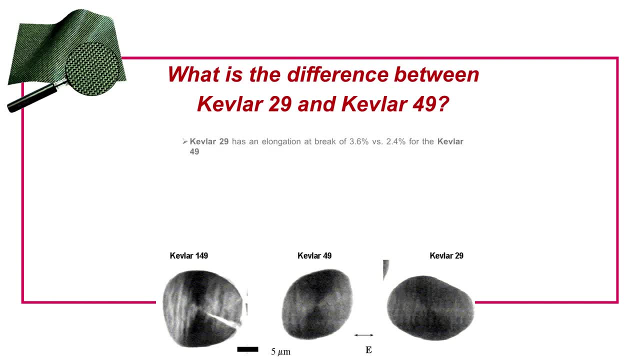 Now, what is the difference between Kevlar 29 and Kevlar 49?? So Kevlar 29 has an elongation, Kevlar 29 has an elongation- Okay, so breaking at 3.6% versus 2.4% of Kevlar 49, and which has on a modulus of elasticity. 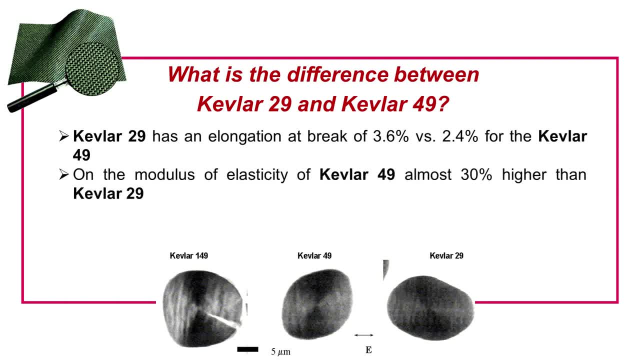 of Kevlar 49,, mostly 30% higher than a Kevlar 21.. So the higher level of Kevlar properties observed that not only at a higher temperature but also at a low Arctic temperature. So these are the